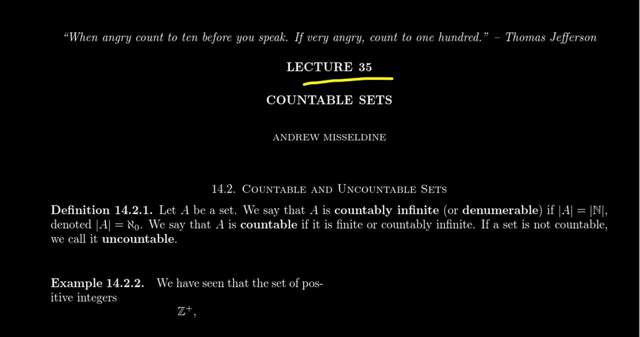 So we've talked about this in lecture 34, and we discovered, looking at power sets, of infinite sets, for example, that not all infinities are created equal, That is, there are some that are bigger than others. In this lecture, we're actually going to explore the smallest type of infinity. 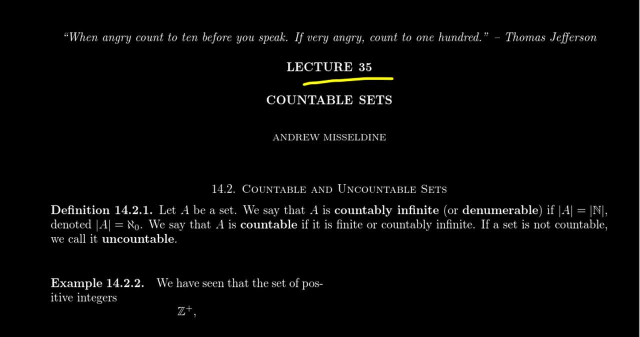 so-called countably infinite sets. all right, So let's get to the titular topic for this lesson here. Let A be a set. We say that A is countably infinite, or some people use the word denumerable here- if the cardinality of A is the same as the cardinality of the natural numbers. 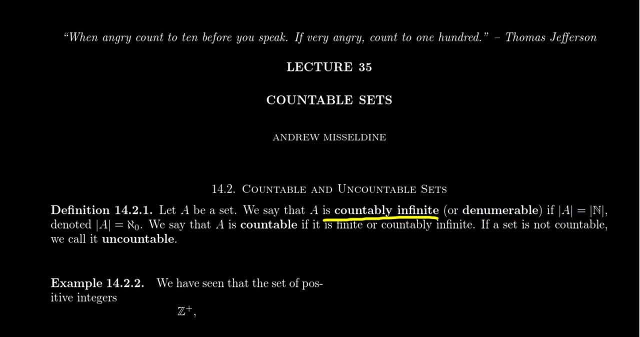 And in that situation we say- we denote this- that A is countably infinite by saying: the cardinality of A is equal to alif-naught. So this symbol right here is actually a Hebrew letter. here It's pronounced alif and you know it's kind of like alpha, but it's the. 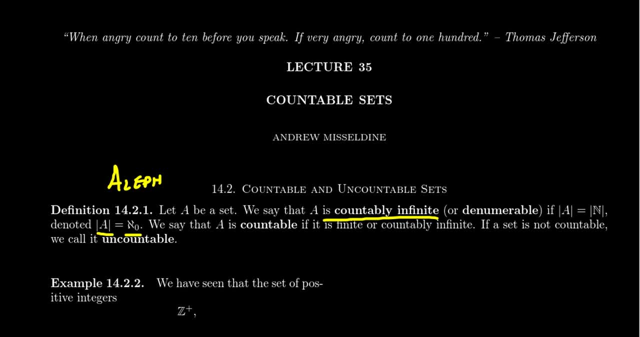 Hebrew version of an. A, I believe- And if I misspeak at all, I'm not the expert of the Hebrew alphabet or anything like that- But alif-naught is the symbol we use to denote the cardinality of countably infinite sets. 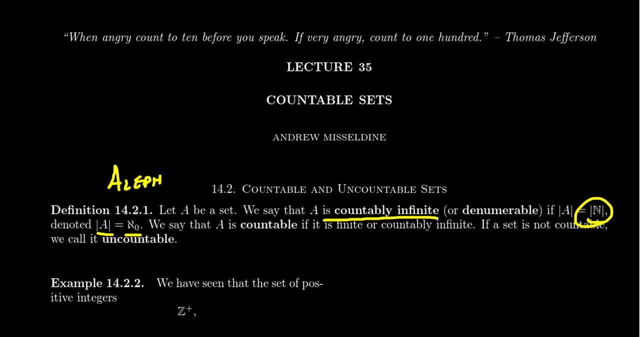 So these are sets that have the same cardinality as the natural numbers. We say that a set is countable if it's either finite or has or is countably infinite. And if a set is not countable, we say that it is uncountable. Now I do have to caution you that in different mathematical text 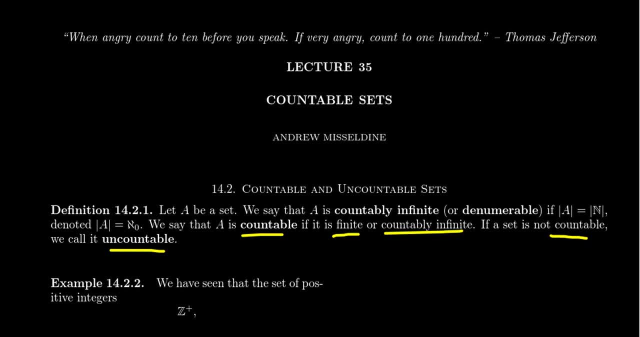 they can use these words slightly different. For example, when someone says denumerable, they might use that as a synonym to countable, as we've defined right here, And some people use countable to mean countably infinite and not finite. So you have to be very careful what 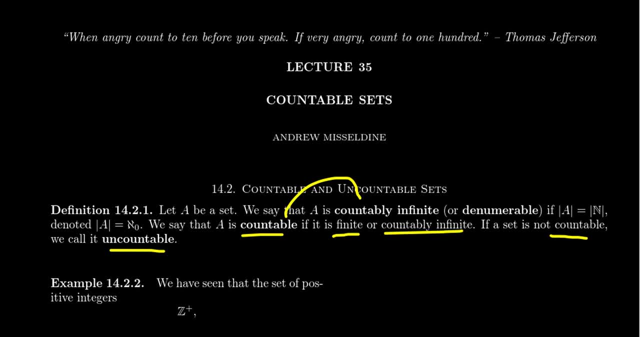 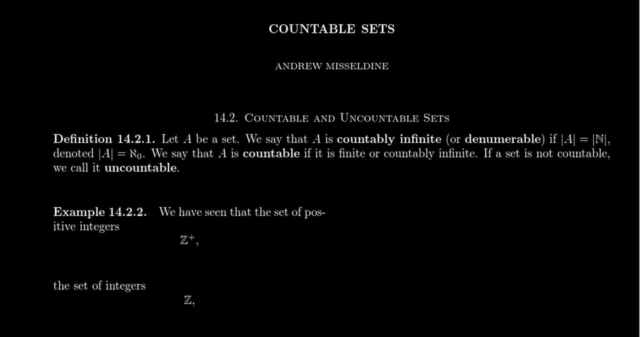 these words mean In our lecture series? countable means that it's finite, or countably infinite. and countably infinite means you have the same cardinality as the natural numbers. Now, clearly, the natural numbers have the same cardinality as themselves. So the natural 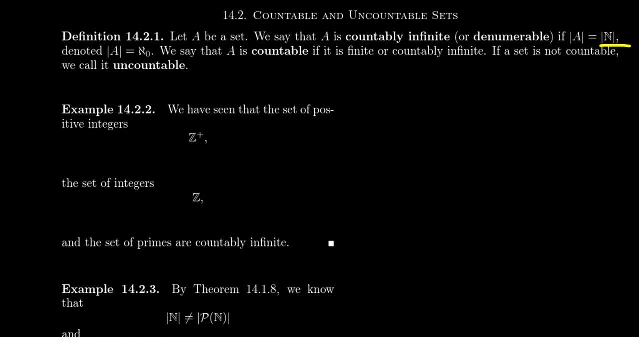 numbers are a countably infinite set. In the previous lesson, lesson 34,, we showed that the positive integers have the same cardinality as the natural numbers. So we have to be very careful between the natural numbers. We came up with a bijection in that situation between the two And 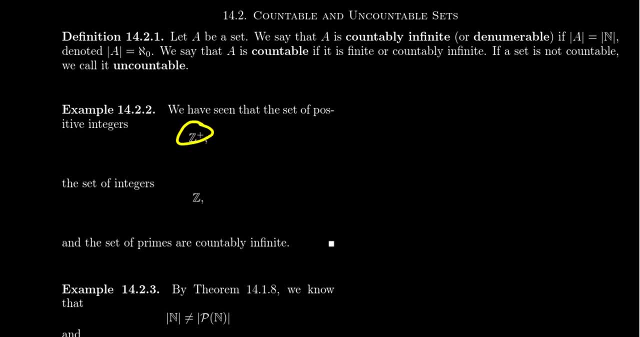 therefore the positive integers gives us a countably infinite set. We also showed that the set of integers positive, negative or zero has the same cardinality as the natural numbers, So this is also a countably infinite set. We also looked at the set of prime numbers and showed: 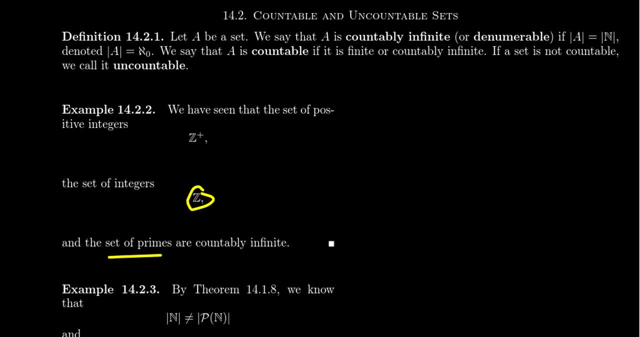 that they are countably infinite. In fact, we made an argument with regard to the primes there that if you take any subset or any infinite subset, you're going to get a set of prime numbers, So this will likewise be a countably infinite set. That also applies to the integers as well. If you 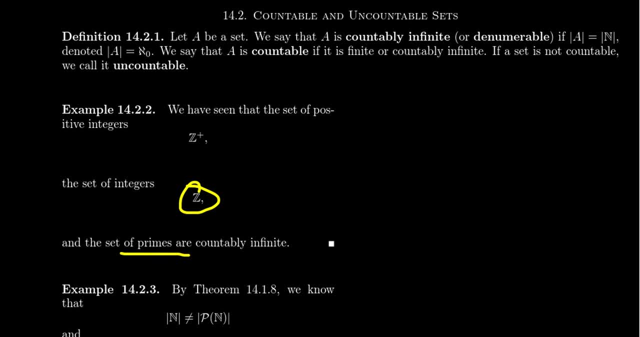 take any infinite subset of the integers, you can actually get a. you will get a countably infinite set. So, in particular, every subset of the natural numbers is countable. Likewise, we can actually argue that any subset of a countable set is countable. but we'll get to more of that in a 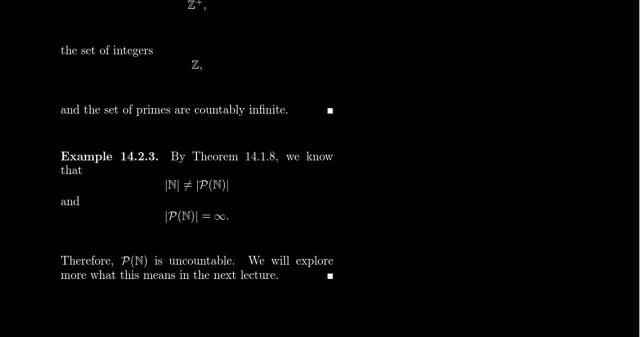 little bit All right Now. we also talked about in the previous lesson that if you have a set of set x, that the power set, that is, the set of subsets of x, has a different cardinality than the set itself. So if you apply that to the natural numbers- the natural numbers, which is of course- 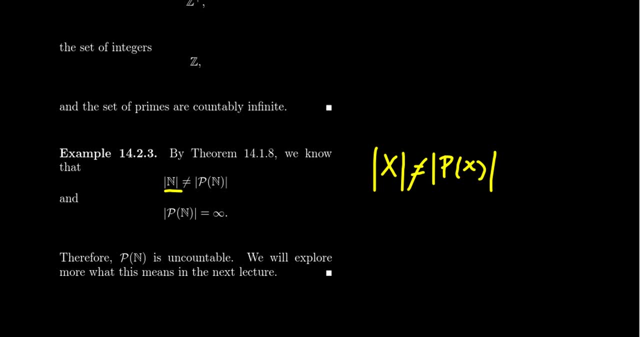 is countably infinite, it does not have the same cardinality as the power set of natural numbers, which the power set of natural numbers itself has to be an infinite set. And therefore, since this is an infinite set, it's not finite and it doesn't have the same cardinality as the set of 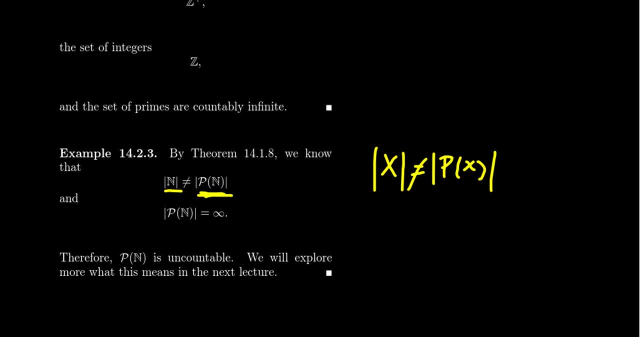 cardinality as the natural number. so this is an example of an uncountable set. so the power set of the natural numbers is an uncountable set and in the very next lesson we'll talk some more about this set. in this lecture i want to explore countable sets, for example. why do we call them? 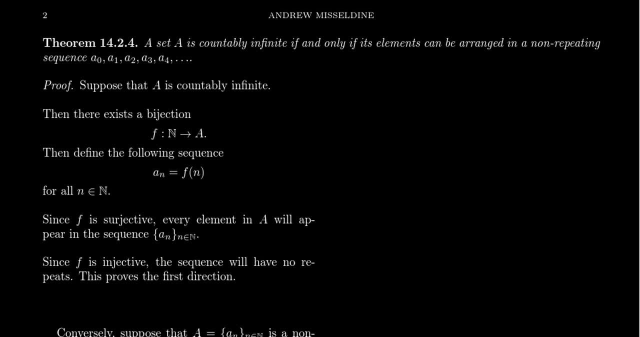 countable sets in the first place. so a set a is countably infinite if, and only if, there exist- uh, there exist- elements, that is. that is this i should say: the elements of the set can be arranged in, not in a non-repeating sequence, so there's some a0, a1, a2, a3, a4, a5, etc. and every term inside. 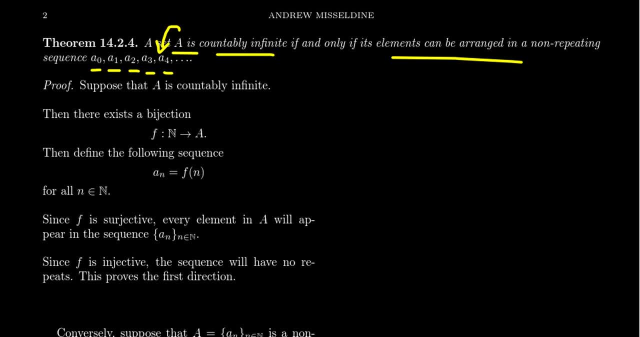 of the set shows up in this sequence once and only once, that makes it a countably infinite set. these two notions are exactly the same thing. now be aware that if you have a finite set, okay, so you have some finite set. we'll call it b for a moment now, because it's 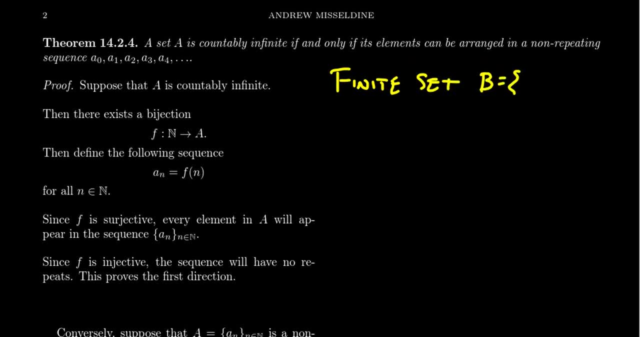 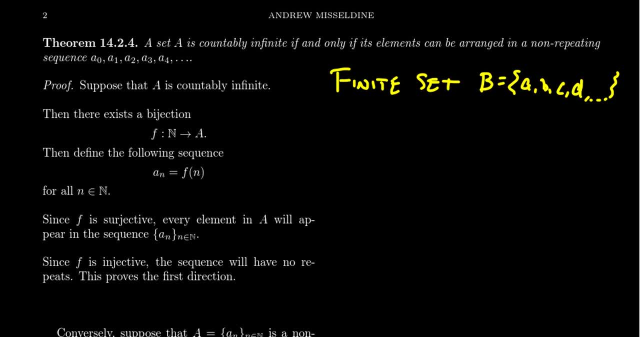 stops does stop after a while, and so you, of those finite elements, pick one of them and we can basically label that the zeroth element, b0. then grab another element that you haven't grabbed already. call that one b1, grab another one, b2, b3, etc. until you get to the end of your list, say bn. 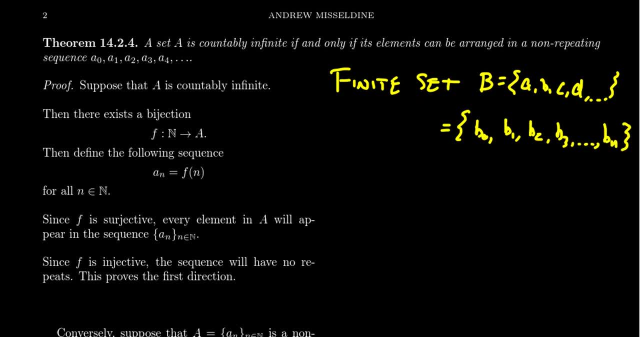 or something like that. if your set's finite, we can, then we can associate, uh, each of these elements with a natural number, because, after all, if it's finite, there exists a bijection from b into the set: zero, one, two, all the way up to n. uh, the way i've written it, i'm assuming that, uh, the 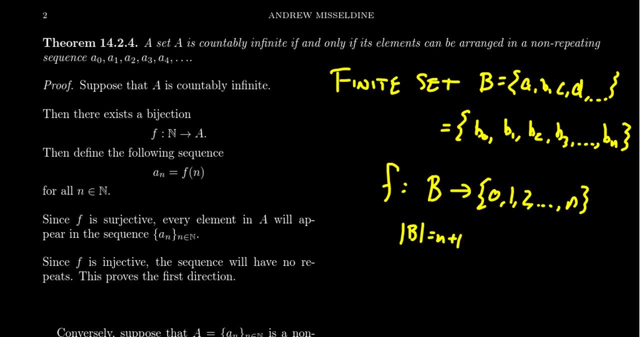 cardinality of b is n plus one. no, no big deal there. but because there's a bijection between the set, the finite set, to this some set like this: you can then use the inordinate of b to the inordinate of b and you can then use the inordinate of b to the 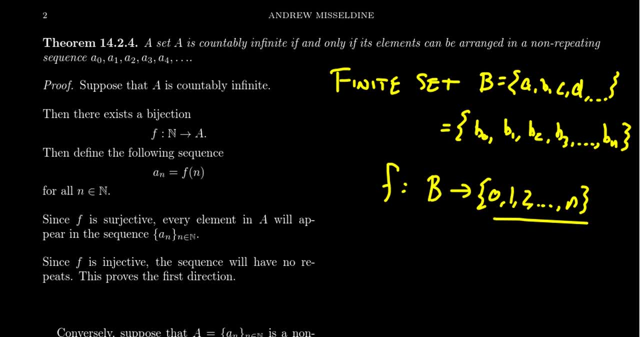 inverse, to provide a labeling like: oh, there's a b0 element, a b1, a b2.. You can list each of these elements, And so you can count them. There's a first element, a second element, a third element, And if you want to start counting at zero, that's fine too, No big deal. 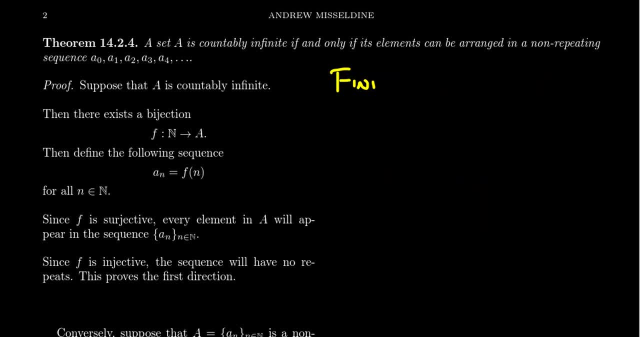 We're saying that for countably infinite sets we can do the same thing, And therefore a set is countable if it's finite or countably infinite. And so the moral of the story here is that a set is countable if you can list every element for natural numbers And then for the 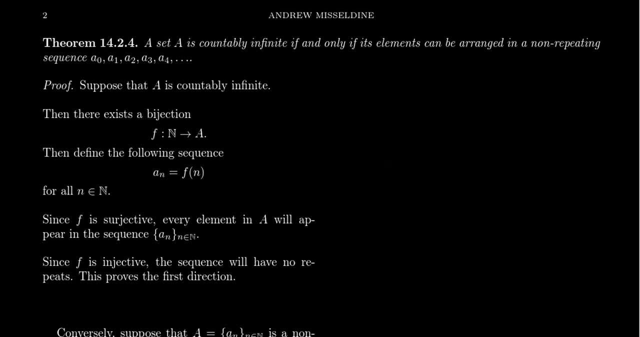 infinite case. it never stops, mind you, But that's fine. So let's prove this. This is an if and only if statement, So we have to prove it in both directions. So let's first assume that a is a countably infinite set. Well, if it's countably infinite by definition. 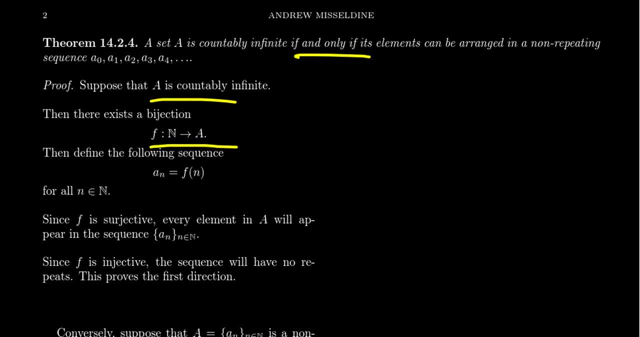 there exists a bijection, which we'll call it f, from the natural numbers into a And that bijection, if we call it f, then we can define the following: I'm going to define a sub n to be the image of n under this map f And therefore this is an. 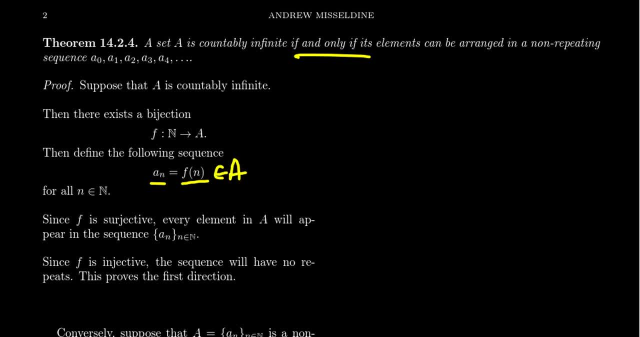 element of a. Since the map is surjective, every element of a appears in this list of numbers, It appears in this sequence, And so of course we can write this: a0, a1,, a2,, a3,, a4,. 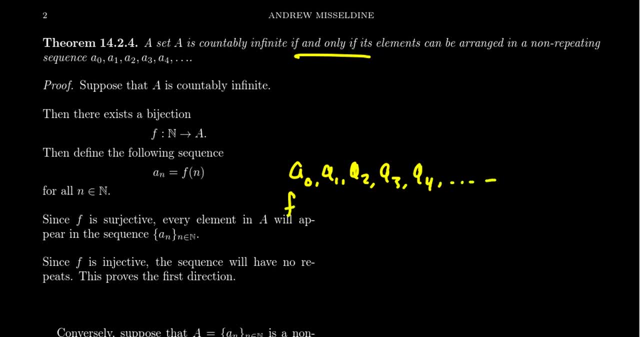 etc, etc. This is just, of course, f of 0,, f of 1,, f of 2,, f of 3,, etc. That's all that this is. These terms are just the images of the function listed in the order. 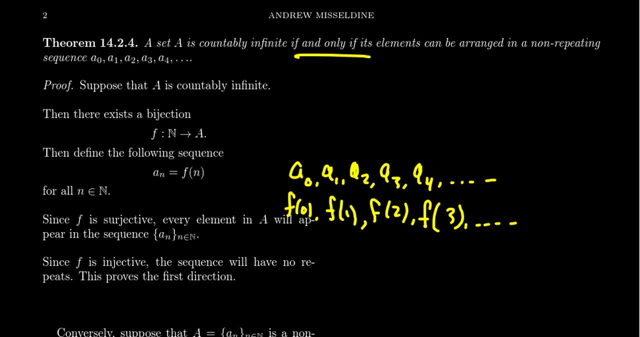 that the natural numbers have 0,, 1,, 2,, 3, 4.. Since this map is surjective, every element of a will appear in this list somewhere, because that's what it means to be surjective. Likewise, 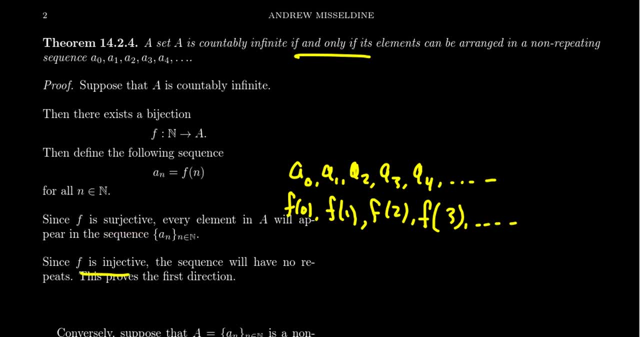 because this function is injective, it's 1 to 1,. this sequence has no repetitions, Because if there were two numbers that were the same, that means we would have two images that were the same and that would violate the injectivity of the function. So because there's a bijection between 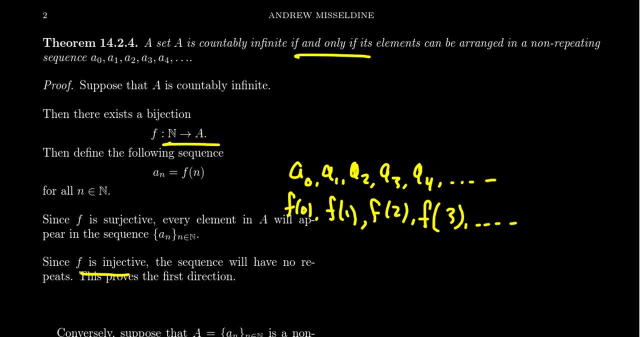 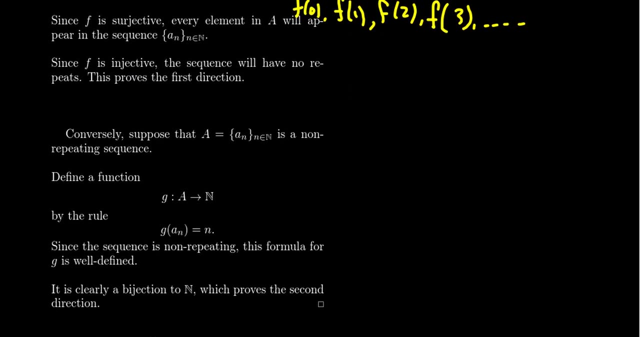 the natural numbers in our set. we can create an infinite sequence using the elements of the set a, with no repetitions, and everyone shows up exactly once. Okay, So that gives us the first direction. Now we want to go the other direction. Suppose that we have that the set a is equal to an infinite 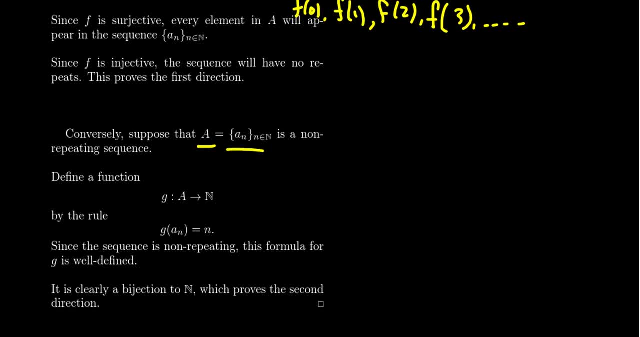 non-repeating sequence, So every element in a can be listed in this sequence with no repetitions whatsoever. We then are going to define a function, We're going to define a function g which goes from a to the natural numbers, such that g of a sub n will maps on to n. Okay Now, since this sequence 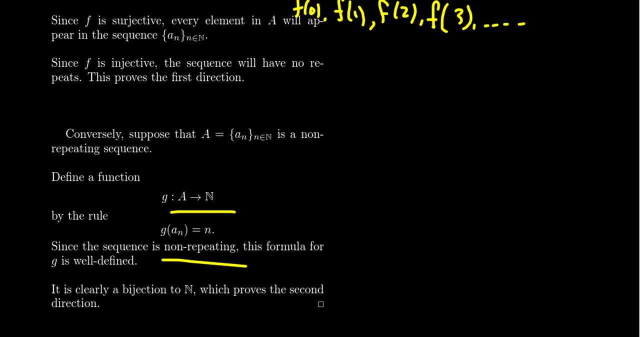 is non-repeating. that means the element a will never show up twice inside this list. So this is a well-defined map. Now, if you had an element, call it x, that was a1 and it was a2, then what is g of x? Is it 1?? 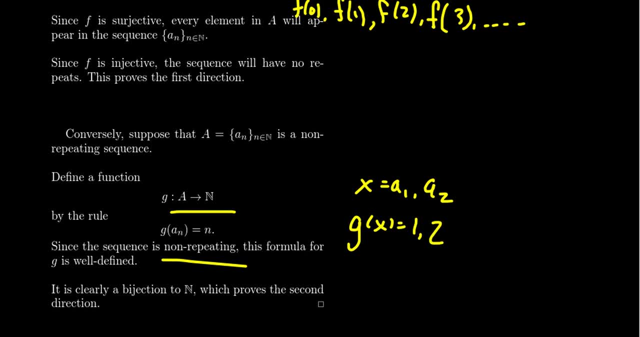 Or 2?? That would be a problem. But since there's no repetition in the sequence, this is a well-defined, well-defined like: if x shows up in the 12th spot, then g of x is equal to 12.. It's a function. 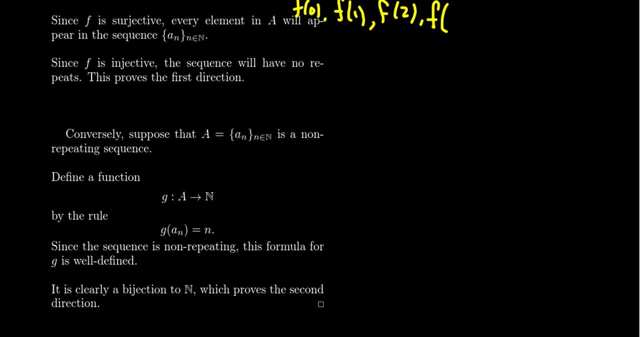 all right, It's well-defined And it's also not too difficult to see that this function is a bijection. It has an inverse, or you can send this thing back like so, And so this is a bijection. So our function- excuse me, our set- since the function is a bijection- is then: 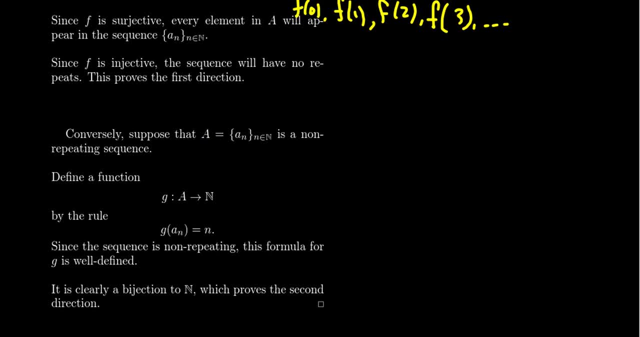 is then countably infinite. There's a bijection going back in the other direction, And so this explains why we call these sets countable. A set is countable if you can list all of them in order right, And it doesn't matter what the order is, because this function kind of places an order on 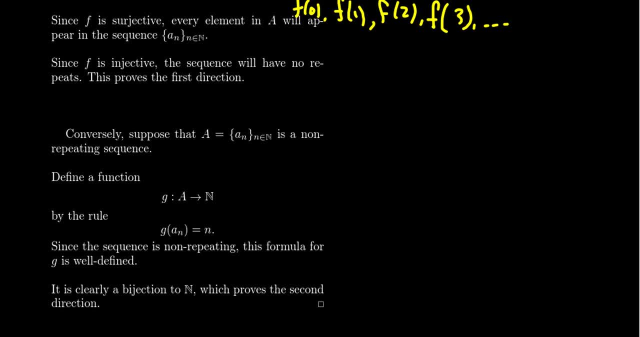 it. It doesn't matter what that order is, but every element can be listed. You can count all of them. That's where this word denumerable comes from. You can enumerate every element inside of the set there. I also want to make mention that in this theorem we talked about 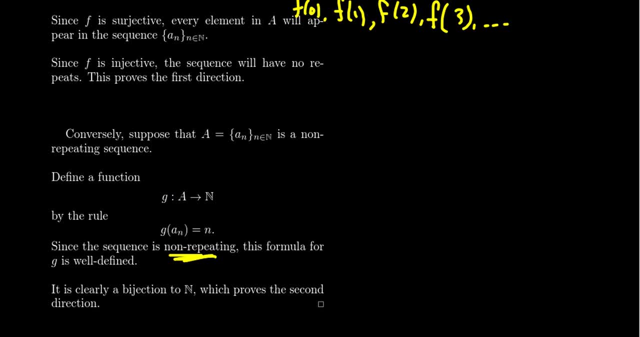 non-repeating sequences. If you have a sequence where everything is listed and there are repetitions, you can just remove the repetitions And therefore every sequence can be restricted to a sub-sequence which non-repeating elements? If again there are any repetitions, just throw. 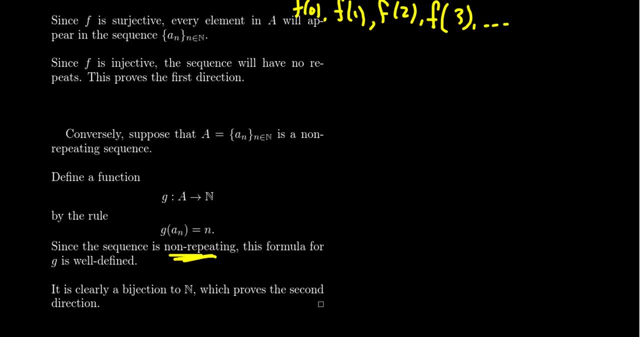 them out. Now, sure, when you restrict it, maybe it's no longer a infinite sequence, Maybe it's just a finite list. That's fine, That still will be a countable set in that situation. So the moral of the story of theorem 14.2.4 here: 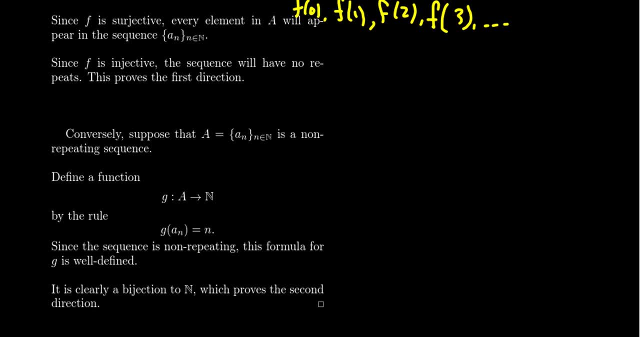 if you can list the elements of the set that makes it countable, And in particular for countably infinite sets. that would be an infinite sequence in that situation. So with that in mind, I want to present to us some corollaries, for which I'm not going to prove. 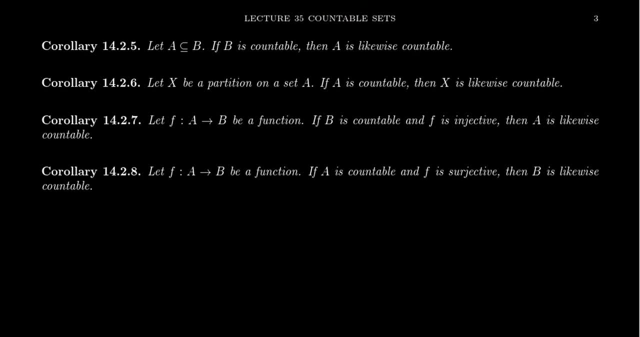 any of these four corollaries. I'm going to leave these as exercise to the viewer here, exercises for my students And honestly, we can prove each and every one of these using this listing condition that they're countable sets there. So I'll give you some hints on how you 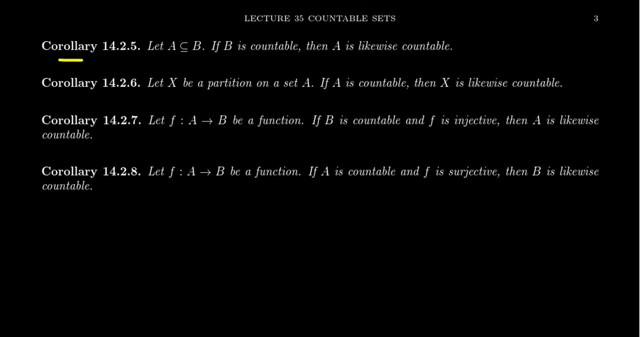 corollaries here. Corollaries because these are consequences of the previous theorem we just proved. So imagine: we have a subset, So A is a subset of B. If B is countable, then likewise A is countable. And how could you argue this? Well, since B is countable, 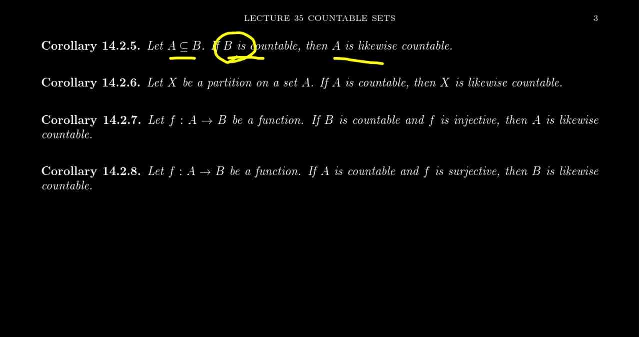 you can list each element here, Since A is a subset of B, and you can list every element of B inside of a sequence. you can then think of A as a subsequence of that sequence. So you just all the elements that are in B, that are not in A. that'll give you a subsequence. And now, since 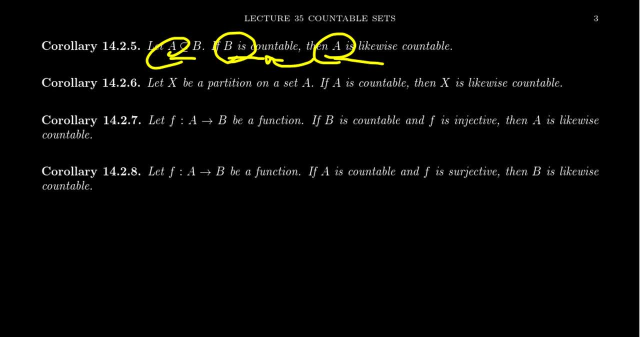 you can list every element in A that shows it's countable by the previous theorem. So I kind of talked about the proof. I'll leave it up to you to kind of write the specific details of that. The next corollary: let X be a partition on a set A If the set which is being partitioned is. 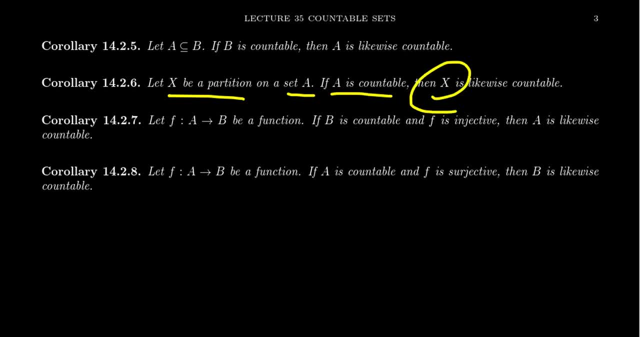 countable, then the partition is countable. That is, if you have a countable set and you place a partition on it, there are finitely many equivalents Classes on that. So another way of saying that is that if you take an equivalence relation on 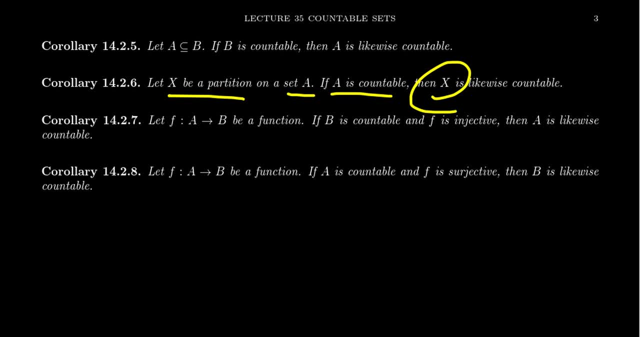 a countable set, the number of equivalents classes is itself countable. All right, I'll leave it to the viewer to check that. Let's get some functions into play here. So if F is a function from A to B and if the codomain is countable and the function is injective, then A is likewise countable. So if 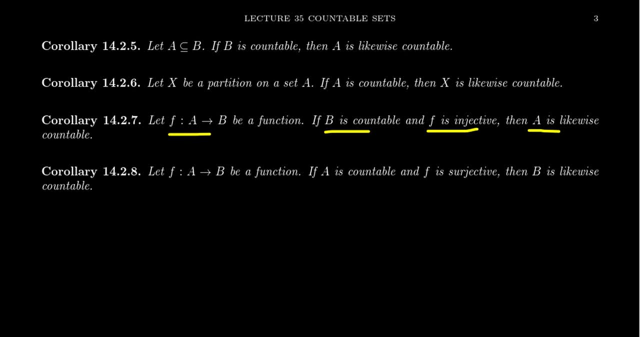 the codomain is countable and the function is one to one, then the domain has to be countable as well. And then the dual argument. there is that, our last corollary: if F is again a function from A to B. 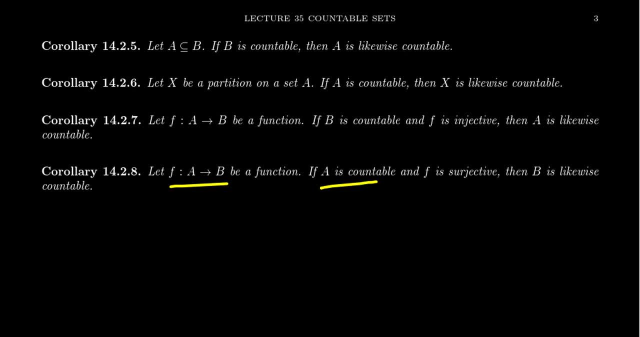 this time the domain is countable and the function is surjective, that is, the functions onto- then the codomain has to be countable as well, And so, again, I'll leave it up to the viewer here to prove all these results. But these are very simple results that come from the theorem. 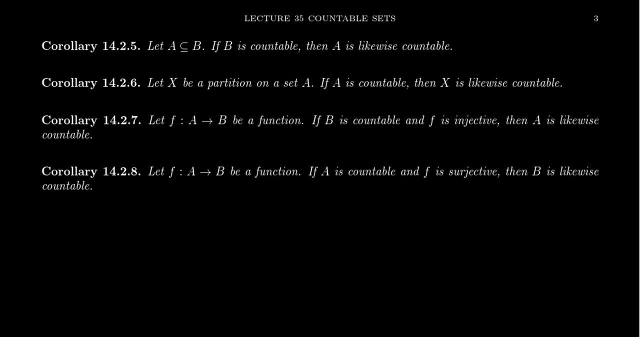 we just proved, If you can list all the elements that makes it a countable set. We kind of talked about how to do that in the last corollary, but if you can list all the elements, that makes it a countable set, And so again I'll leave it up to you to kind of argue this one here Now. 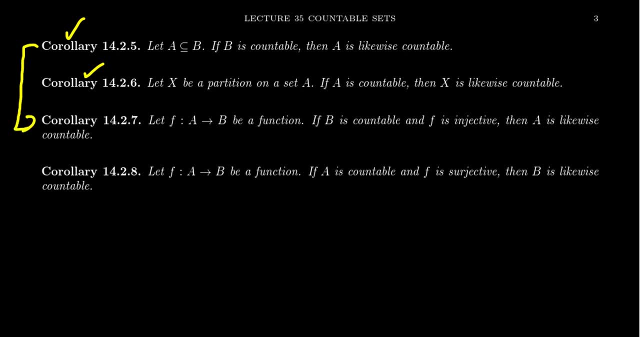 I mentioned that if you have this one, you can use that to prove this one, And if you have this one, you can use that to prove this one here, But I'll let you fill in the details of those. We're going to look at some harder ones here. So I want to talk about how countable sets interact with the. 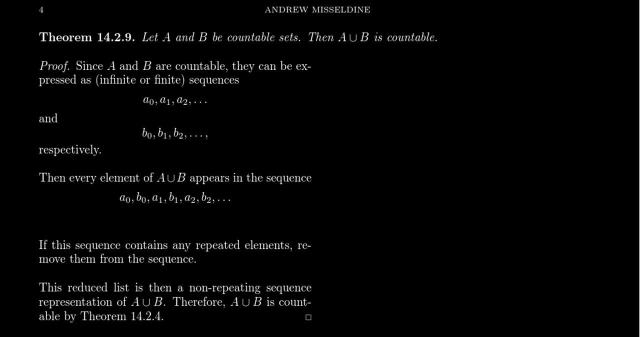 operations of sets that we've already been talking about, Like, for example, if you have two countable sets, what about their union? And it is a fact that the union of two countable sets will be countable itself. Now I don't need to say much about intersections, because if you're 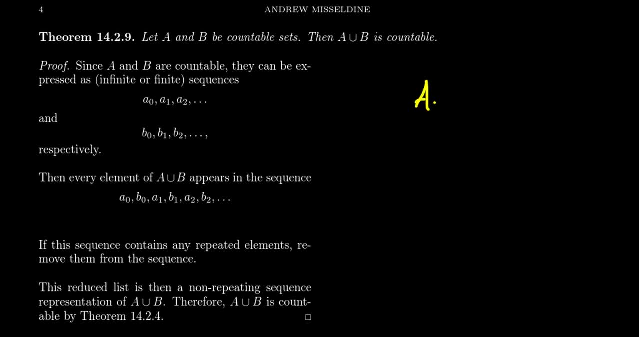 like: oh, A and B are countable, what about A intersect B? Well, if you take A, intersect anything. if A is countable, it's a subset of A which was countable by assumption. So by the previous corollary we had just talked about, all subsets of countable sets are countable, So intersections. 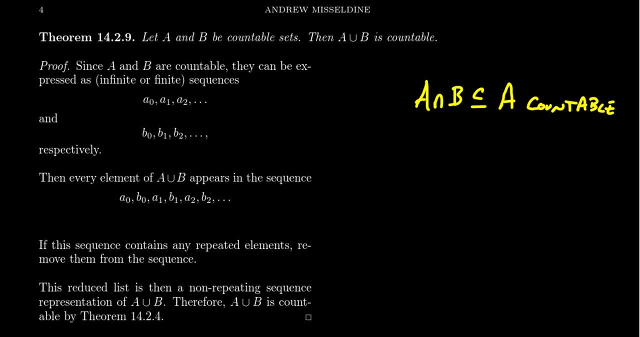 are too easy, Like: if you intersect two countable sets, you're going to get something that's countable. Honestly, if you intersect a countable set with anything, you'll get something. countable. Unions, on the other hand, a little bit harder, because you're getting something 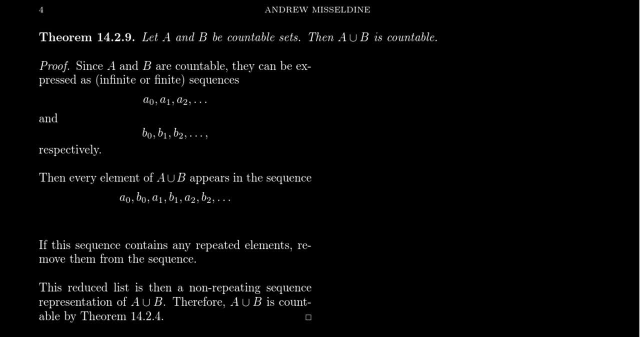 bigger. How do I know? the bigger thing is still countable. Like what if you take two sets and you make it so big that you can't count it anymore, right? Well, let's look at the proof of this thing. Suppose A and B are countable, Then that means our sets A and B can be expressed as: 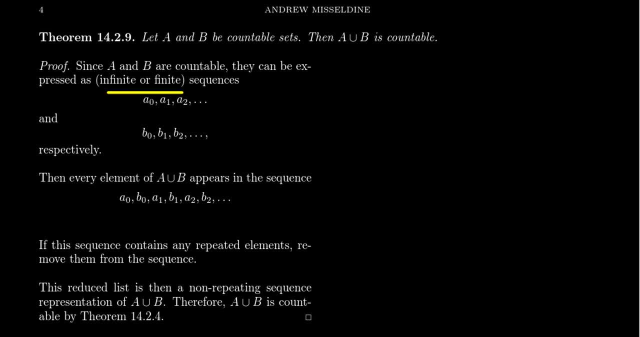 sequences. Now, those sequences could be infinite or finite, I don't care. We get two sequences, So all the elements of A will look like A0, A1, A2, keep on going. If it's finite, this will eventually terminate. If it's infinite, it'll go on forever. Not a problem. Do the same thing for B. 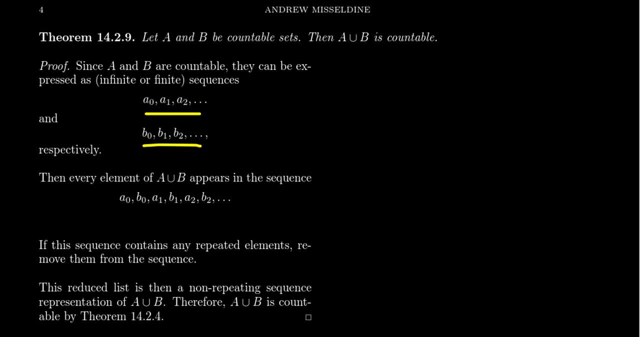 Every element of B can be listed: B0, B1, B2,, B3,, B4, keep on going. Okay, Then, in order to show that A union B is countable, all we have to do is argue that the elements of A union B can themselves. 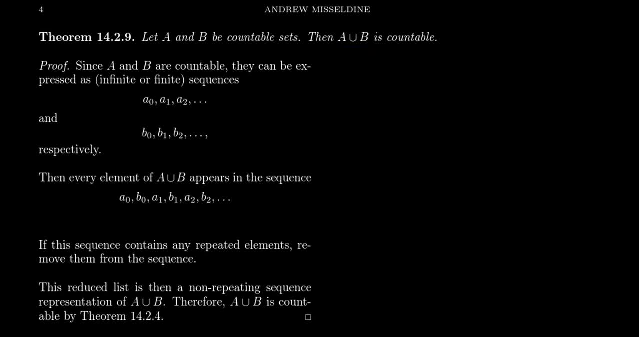 be listed, And we're going to list every element of A union B using the following strategy: We're going to do A0, B0, A1, B1, A2, B2.. And then we're going to continue to alternate between the two. 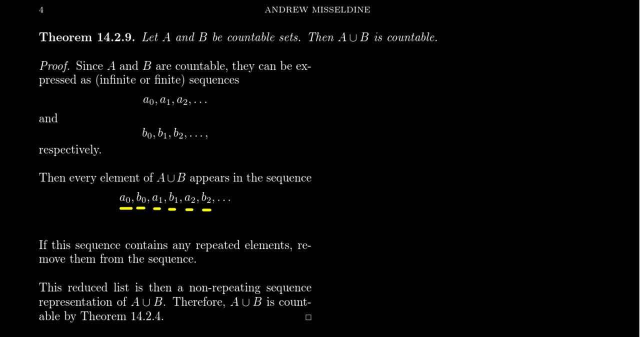 elements. The next one would be A3, then B3.. Then A4, then B4, then A5, then B5, et cetera, et cetera. So we're just going to, we're going to. 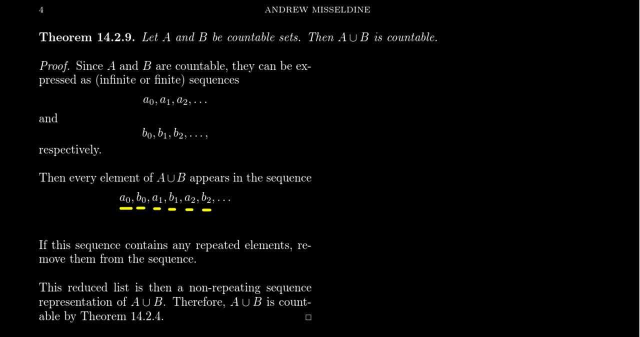 mesh the two sequences together, interlocking them like so. Now, if any of the sequences are finite, then you can stop alternating. Once you've exhausted all of the elements from A, then just continue to list elements for B forever onward. That's how we're going to handle that. 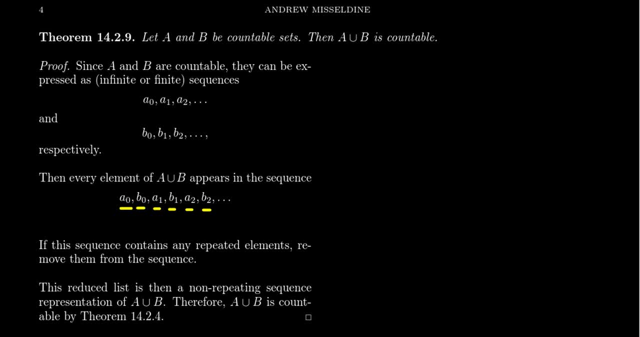 Or same thing: If B is finite, then once you've reached the end of B, you can stop. you can stop your zipper, Cause that's the idea We're trying to like: zipper these two sequences together. Now, if you have a sequence that's finite, then you can stop your zipper. 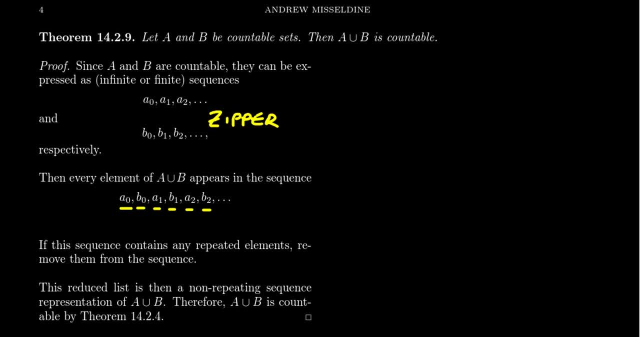 If one of them has more teeth than the other, then just stop the zipper process at that moment. If they're both finite, this will be just fine. Now we're taking a union. It's very possible that the elements of A do overlap with the elements of B. There could be an element that's 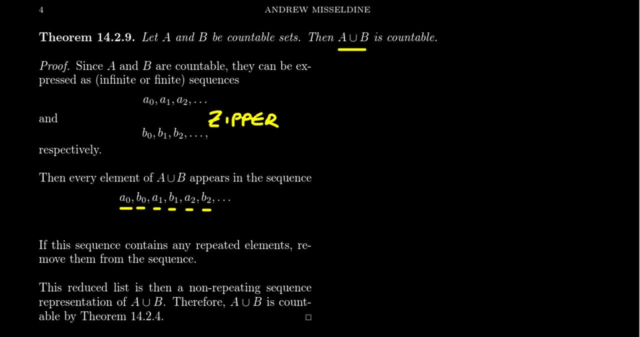 in A and B like. so, As such, this sequence very likely could have repetitions inside of it, But if there's any repeated elements, just remove them after the first appearance. So we have this sequence. If there's any repetitions. it's like: oh, A zero is equal to B two, which is like: oh, just remove B two from the list. 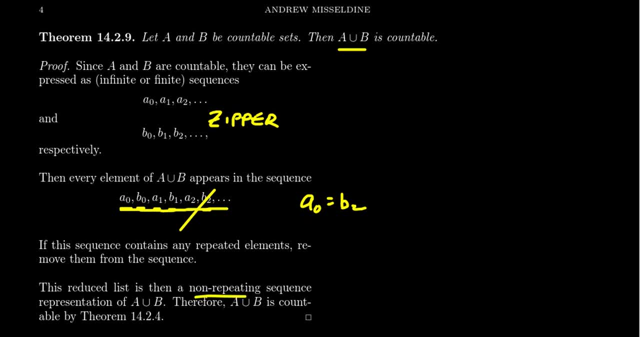 We will then get a non-repeating sequence of elements, And every element of A union B will be in this list, because if it was in A, it showed up here, Thus it'll show up there. If it was in B, it'll show up here and thus will also show up there, And, as such, 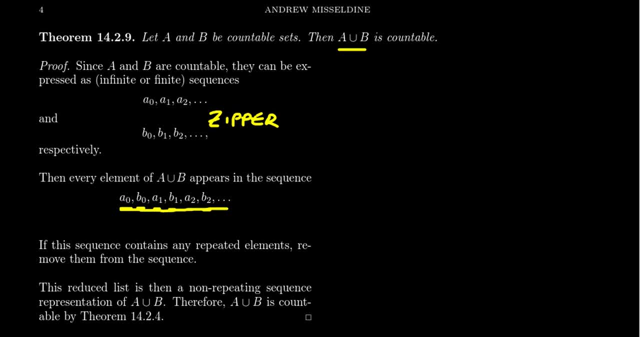 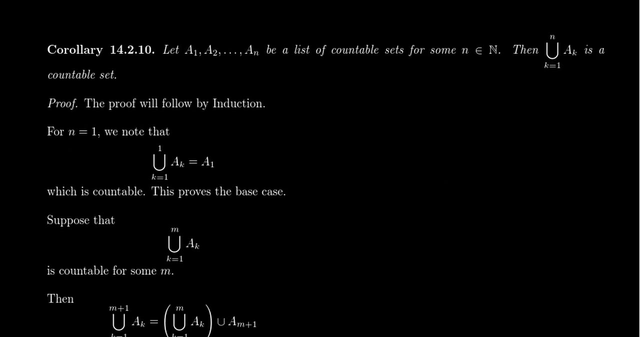 every element of A or B will show up eventually, And so we've now constructed a non-repeating sequence of elements from A union B. Therefore, A union B is a countable set. Now, if we apply induction here, we can actually show that an arbitrary union. 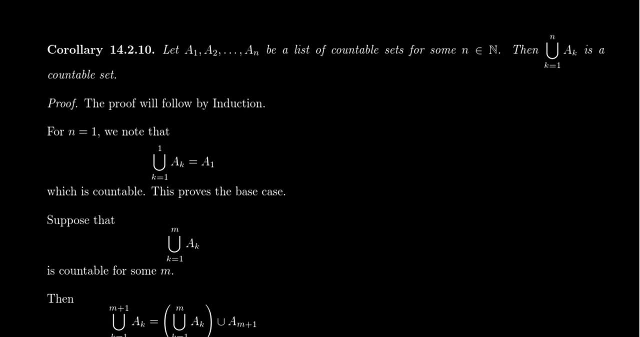 that is, a finite union of countable sets, is likewise countable. So this is a corollary to the previous theorem we just talked about. So A1, A2, up to AN, these are each countable sets for some natural number, N. Then the union where K ranges from one to N of A sub K. 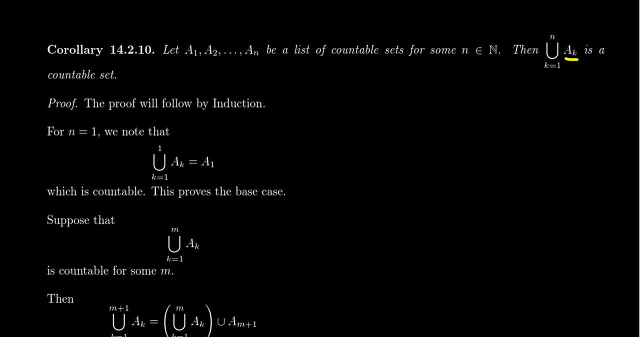 this is itself a countable set, And we can prove this by induction. So for induction we have to do the base case. So suppose N equals one. Note that if you take the union of K equals one to one of AK. this is just A1 itself. 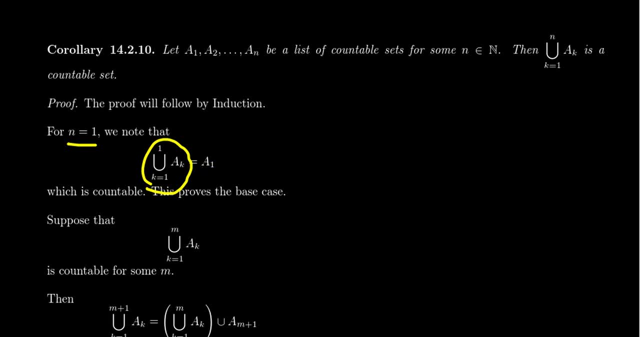 And A1 is a countable set. Now, I guess technically the base case should start off with zero, because that's the first natural number there. And so in this situation, taking the union where you have nothing inside of it, an empty union is actually the empty set itself And, as such, the empty set. 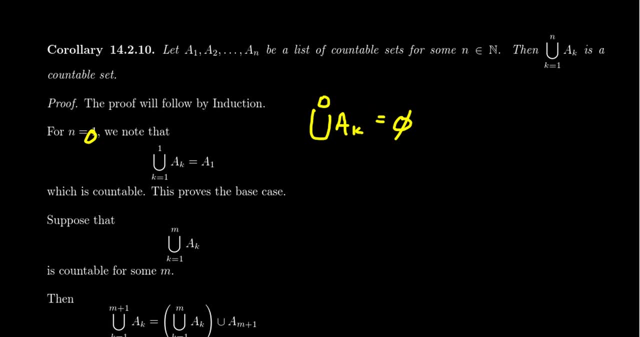 it's a finite set. it's countable, So that would still work. Some people find this a little disconcerting, But if you take the union of K equals one to one of AK. this is just A1 itself. But we should be very comfortable with these trivial zero cases. So really the base case. 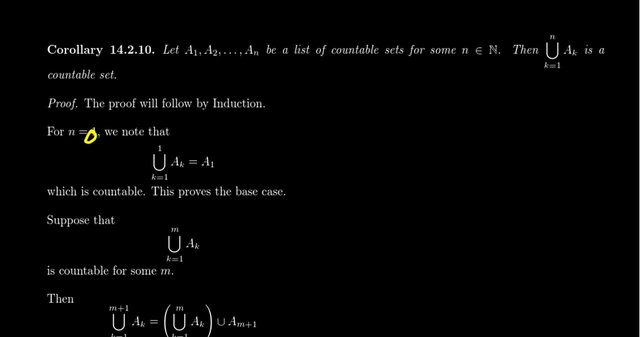 should be N equals zero. But if you're uncomfortable with that because like an empty union, oh no, then take N equals one and you can do your base case there. Not a big deal. An empty union would be the empty set, because the empty set acts like the identity for unions. Okay, so we get our base. 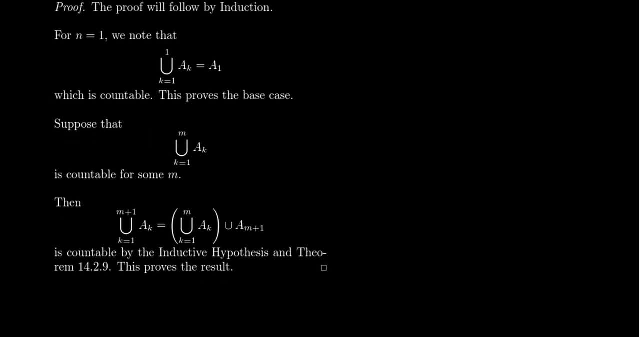 case. So then let's take our inductive hypothesis. So suppose that the union where you take K equals one to M, where M is some positive number, and you take the union of K equals one to M, to take the union, the M-fold union of AKs, that this is a countable set. Okay, so then that's our 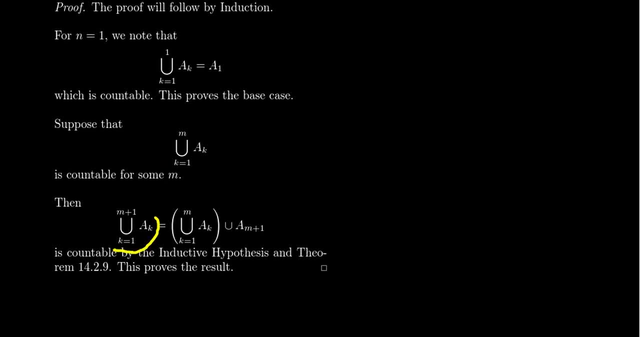 inductive hypothesis. Assume, no, not assume. consider the union where this time we go from K equals one to M plus one. You take the union of all those sets, A sub K. Well, so the only difference between this union and this union is we've now joined on one more set, So we can. 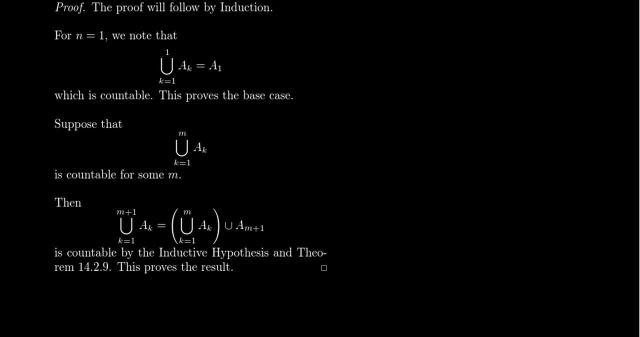 actually decompose this union into the M-fold union of AKs. So that's our inductive hypothesis. Okay, so let's take our inductive hypothesis. Assume, no, not assume. consider the union of K equals one to M. where K equals one to M plus one, You take the union of all those sets A sub K. Well, 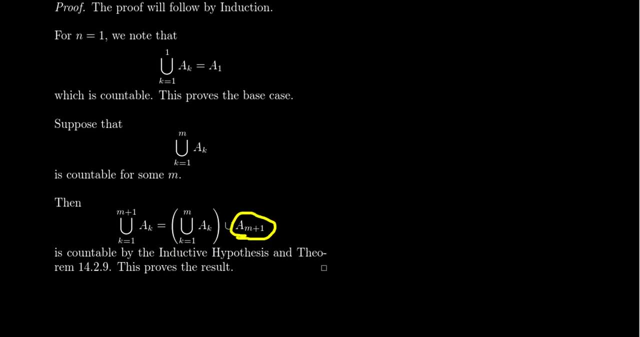 A, M plus one is countable by assumption. That was the assumption of the sets A1, A2, A3, up to A, whatever AN, These are all countable sets. So that's a countable set By our inductive hypothesis. 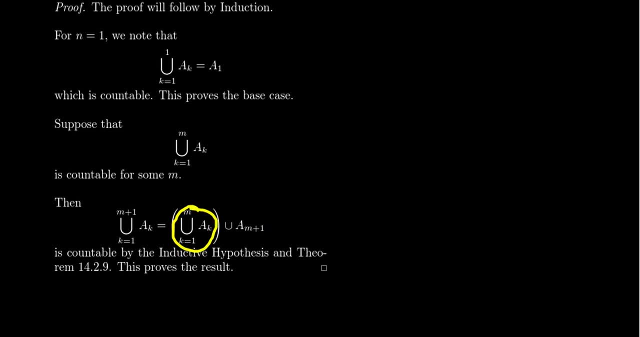 this is a countable set, And therefore the union of two countable sets is countable. That's what we proved previously. So theorem four, three, four, five, six, seven, eight, nine, ten, eleven: 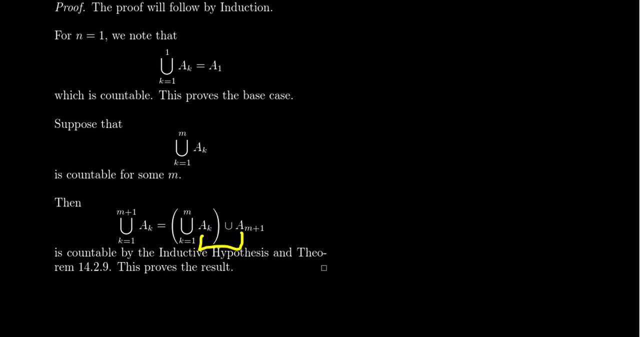 fourteen, two, nine, which is just above on the slide, shows that the union of two countable sets is countable. So therefore this is countable And therefore the result follows by induction. If you take a finite union of countable sets, that is itself countable. Same thing with 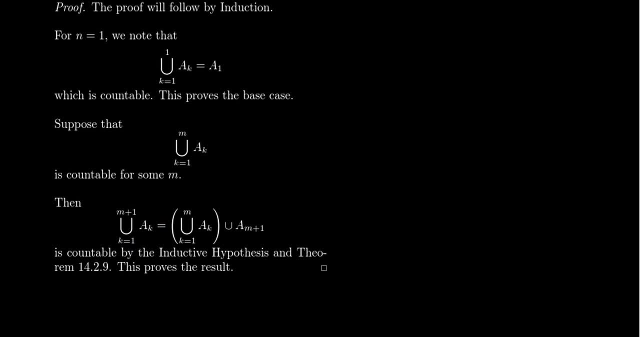 intersections. but that argument's much easier If you take the intersection of A sub K, where K ranges from one to N. I don't need induction there because this is a subset of A sub K. We'll just say it's the subset of A1, right? 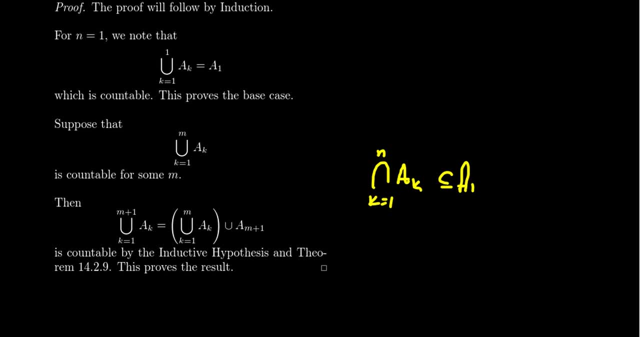 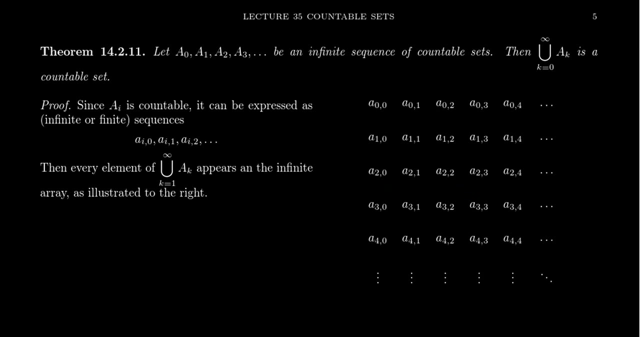 A1 is countable, so this intersection is countable as well. all right, No big deal, not a problem there. Intersections are much easier because subsets of countable sets are themselves countable. All right, What if we take an infinite union of countable sets, That is, 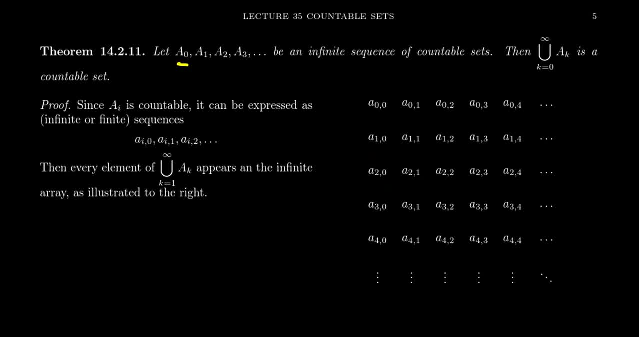 suppose we have an infinite sequence: A0, A1, A2, A3, A4, A5, etc. etc. We have a countable set for each of the natural numbers. We have a countable set for each of the natural numbers. We have a. 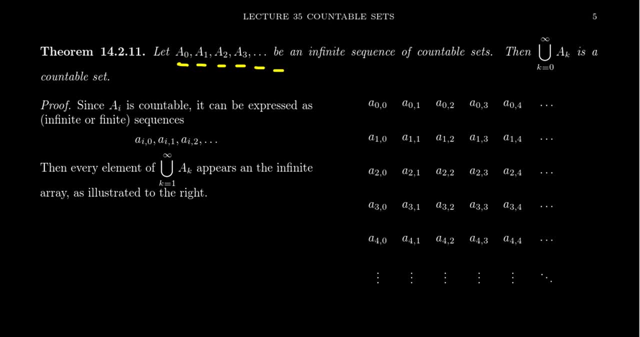 countable set for each of the natural numbers. Each of these A sub I's is a countable set. okay, So then if we take the union where K equals zero to infinity of all of these sets A sub K, if each of the sets A K is countable, then this countable union will also be countable, And I do. 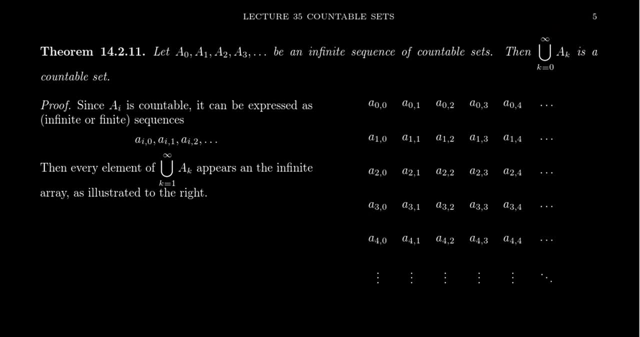 say this is countable union. If you take a union where you take the union of the A sub X's, where X is a, you know an element of the real numbers we're going to see- not yet, but the real numbers- is an uncountable set. If you take an uncountable union of countable 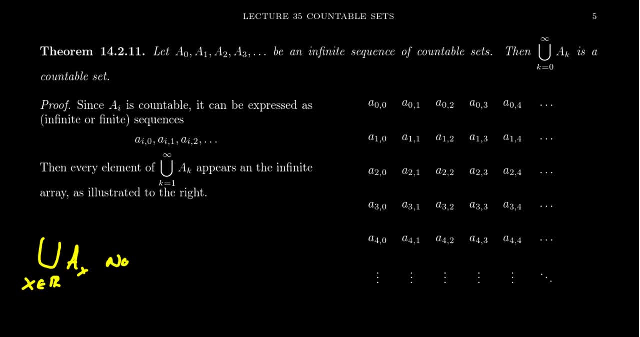 sets, this might not be countable. Not countable- Well, maybe It's hard to say. I mean like if you take, if you take the natural numbers and union and you unite that even on uncountable times because there's the overlap is the whole thing- You can still be countable. It's like 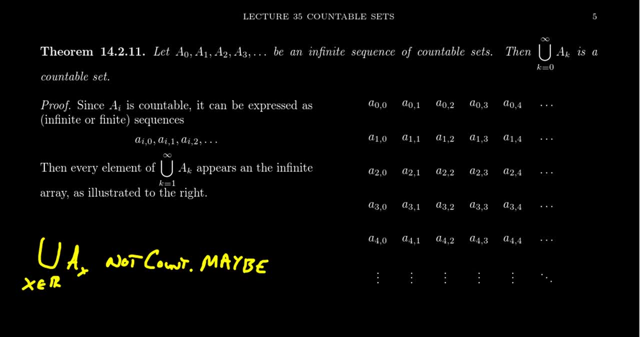 but the thing is, if you take an uncountable union of things- because that when I say an uncountable union I mean the index set of the union is itself an uncountable set- you might not be countable anymore, right, But with regard to the countable unions of countable, 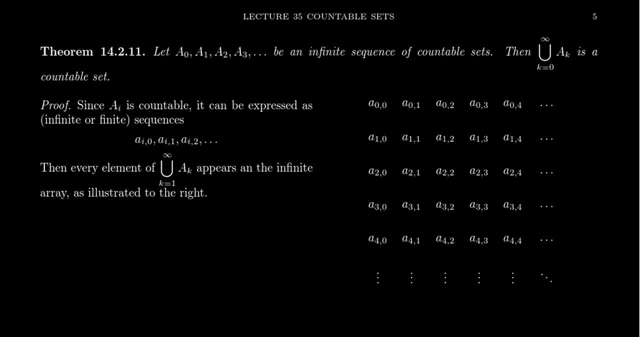 sets. this is in fact always going to be a countable thing. So we've already taken care of the finite case. So to show that a countable union of countable sets is countable, we only have to deal with the union be countably infinite. So there are countably infinite. 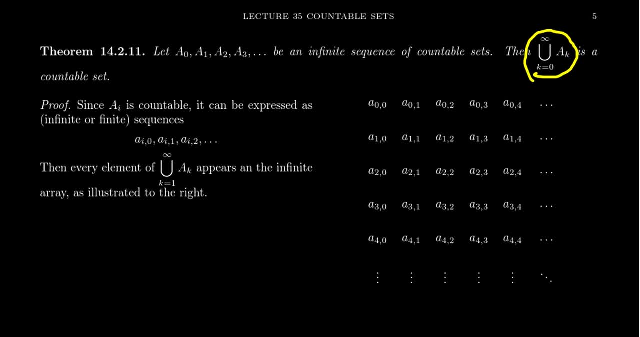 there's countably infinite many sets inside of this union. If each of the sets is countable, this is going to be a countable set, All right, And the way we're going to do this is that we have to come up with a set of sets that are countable. So we're going to do that. So we're. 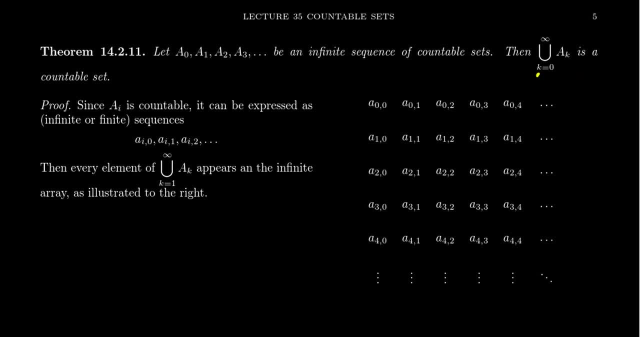 going to list every element in the set in an infinite sequence. Okay, Now, since AI is a countable set, so AI is just one of the sets inside of this list here, since it is a countable set, again, it could be infinite or finite, I don't care. Each of the elements inside of AI. 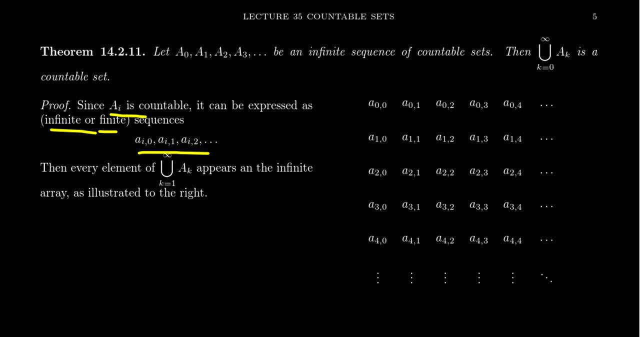 can be listed as a sequence which we're going to use a double subscript to keep track of things here. So the, the zeroth element of AI, we're going to call AI zero. The first element, we'll call it AI two, et cetera, AI three, AI four, AI five, AI six, et cetera, et cetera, et cetera. 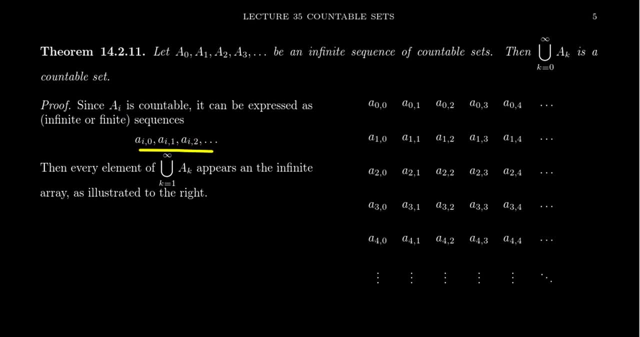 So every element here gets that, And again, if there is, if there's any, if it's finite, this might stop after a while. not a big deal Now. every element in the countable union could be arranged not as a sequence, but actually as a two dimensional array, kind of like an infinite. 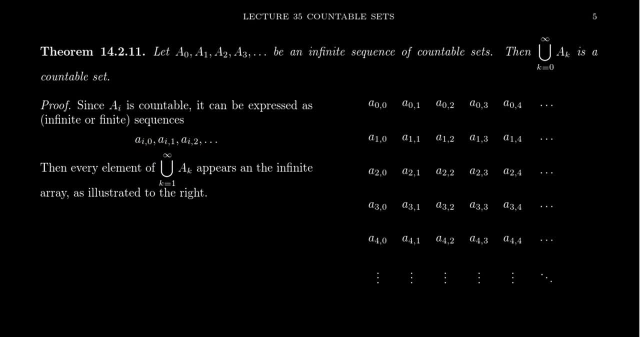 matrix over here, for which the first row of the matrix is the first set, a zero. The second row here will be a two, The next row would be a three, et cetera and et cetera. Okay, So that's how. 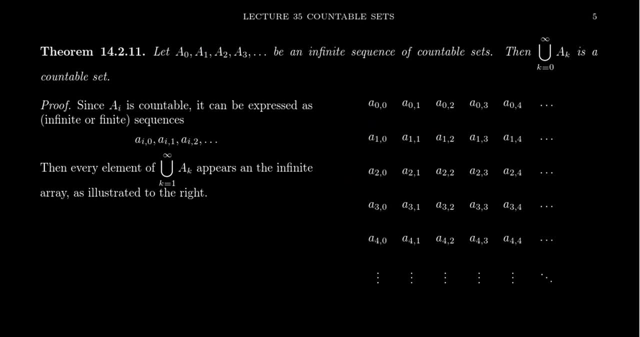 we've done. We've arranged it here, And now every element will show up somewhere in this array. uh, because every element in a zero shows up in the first row, Every element of a one shows up in the next row, Every element of a two shows up in the next row, So every element will show up. 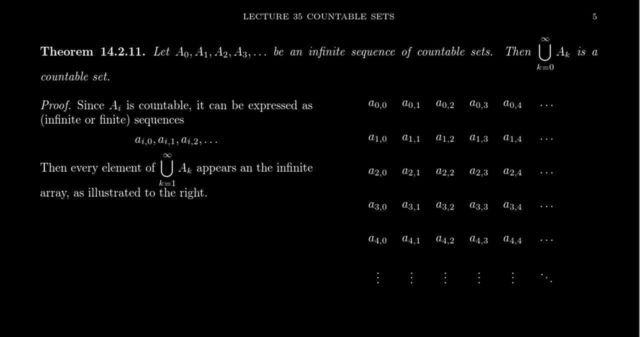 eventually inside of this thing. So, be aware that this two dimensional infinite matrix- well, it's potentially infinite matrix- Some of these rows might terminate after a while and the whole thing might terminate, I suppose, Although we are assuming infinite rows in this situation, the columns might stop after a while. Anyways, every element inside. 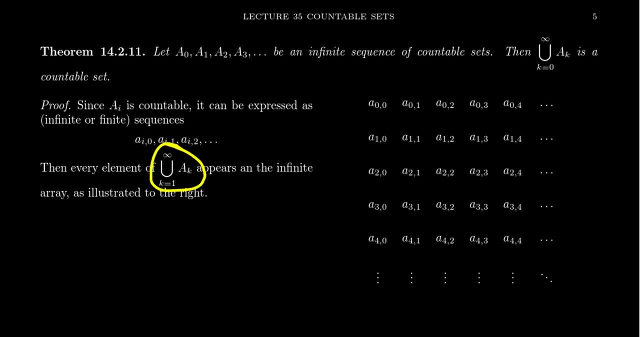 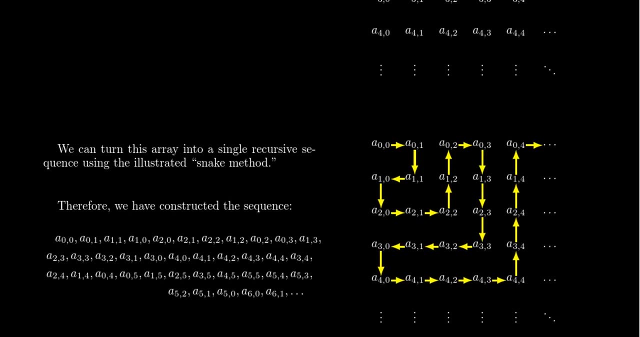 this countable union will show up somewhere in this array. So how do you turn this two dimensional array into a one dimensional sequence? Well, we can accomplish that using what we call the snake method. We're going to have a little sneaky snake that's going to slither through this. 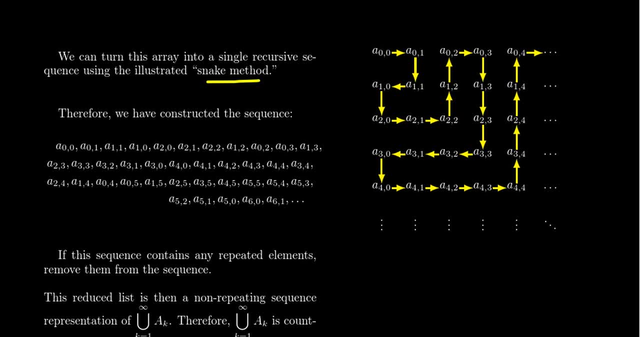 entire diagram Um. to use a calculus analogy. what we are talking about is a space filling curve, Um, but instead of having some type of like continuous topology, um, we're actually talking about a discrete array. So it's a much easier to get a space filling curve, but that's exactly what we're trying to do here. 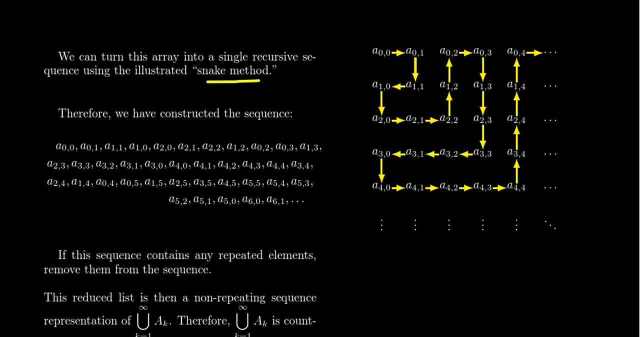 We're going to have a. we're going to make a sequence by snaking through all of it. So what you're going to do is you're going to start with the upper corner, the a zero, zero spot. Then, following this snake, you're going to go to the a one spot, a one, one zero, two zero. 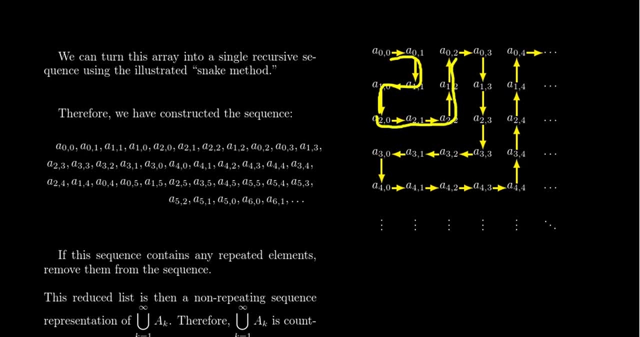 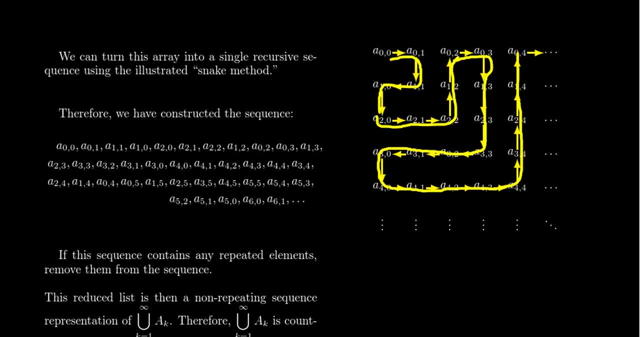 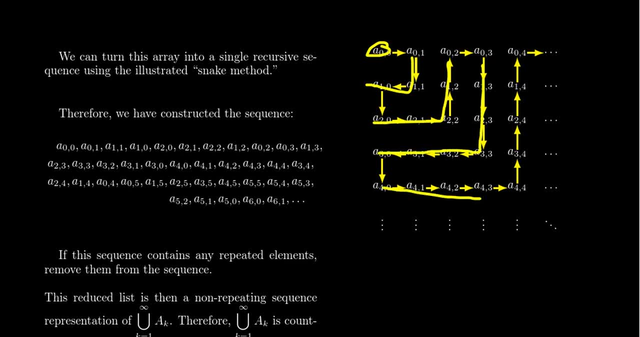 there's this one, there's this one right here, So you have these layers, these L's, shaped objects, inside of the array, And so then what you do is use, transverse each of these, these layers, each of these L's, And once you, once you've finished the layer, you just jump. 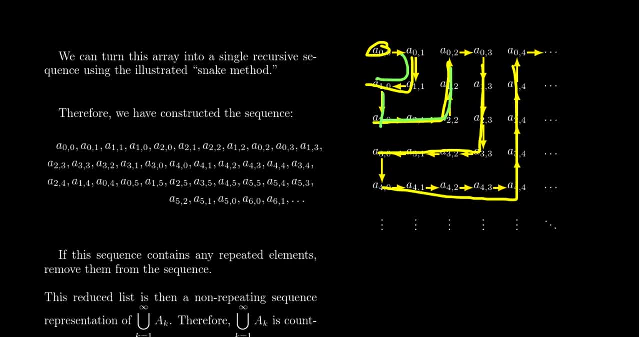 to the next layer and go over. then you jump over, do the next one, then jump over, do the next one. So what we do is we jump here and then we do this layer, Then when you jump down and go to the next, 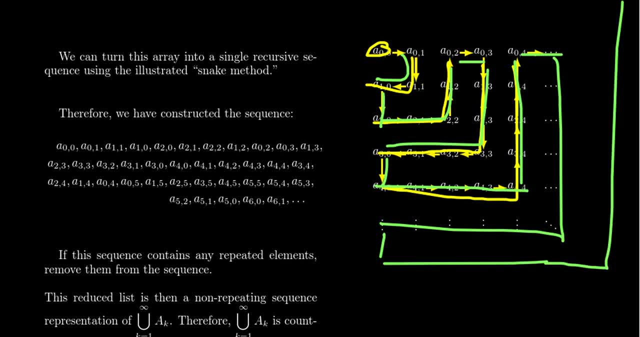 one like so, and you keep on doing this over and over and over again, going towards infinity. Okay, Um, so basically, when you end you, one of your coordinates is going to be a zero. If the second coordinate is zero, then you're just going to increase the first coordinate by one. 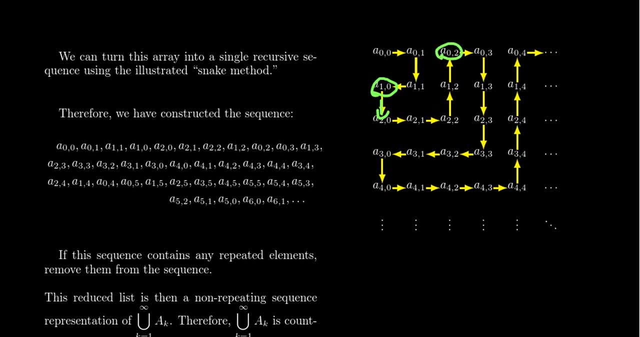 But if you end with the first coordinate being zero, then you're just going to increase the the second coordinate by one. So, like I said, whenever you end a layer, you either you, you end with a zero. one of either the first or second coordinate is a zero. 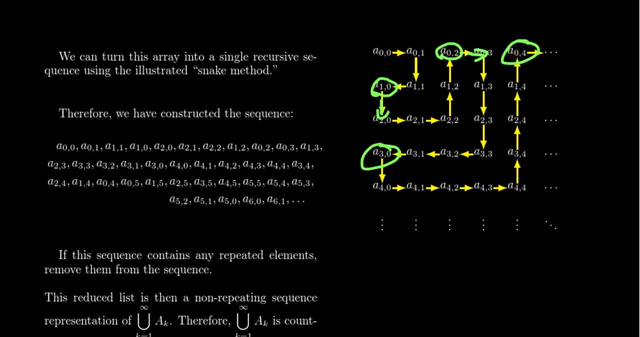 just increment the non-zero coordinates, the next natural number and then continue going through the layers. This snake method will grab everything in the two dimensional array, And so this then turns everything into a sequence, right, So that sequence will look like what I read earlier: Um a 0, 0, 0, 1, 1, 1, 1, 0, 2, 0, 2, 1, 2, 2, 1, 2, 0, 2, 0, 3, 1, 3,. 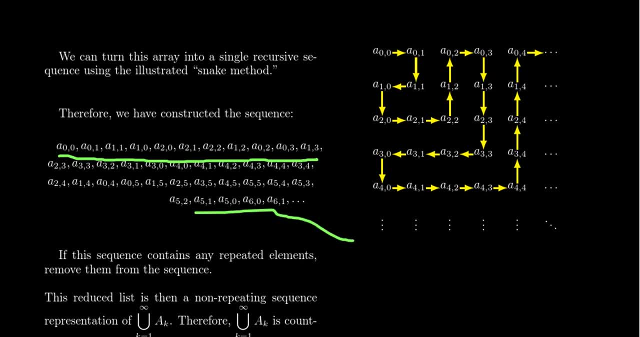 et cetera, et cetera, et cetera. You're going to go all the way through. You're going to grab everything. All right. Now, if there reaches a point where there isn't a number because the list was finite, that's okay. Just skip over that spot, No big deal. If you ever reach a point where 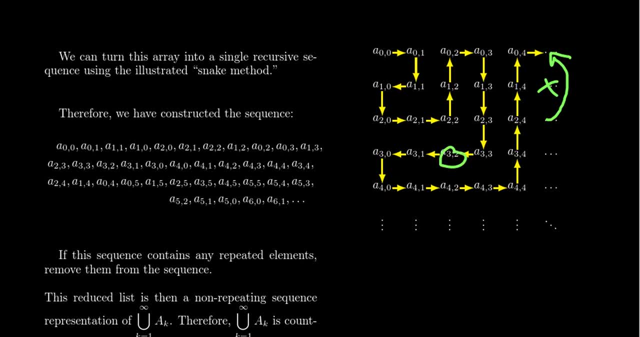 you get a repetition like this number and this number were the same thing. The first time you find it added to the list. The second time you find it, just skip over it. You don't use it. Like I said, if it's finite, if there isn't a spot, if there's a gap, just skip over until you. 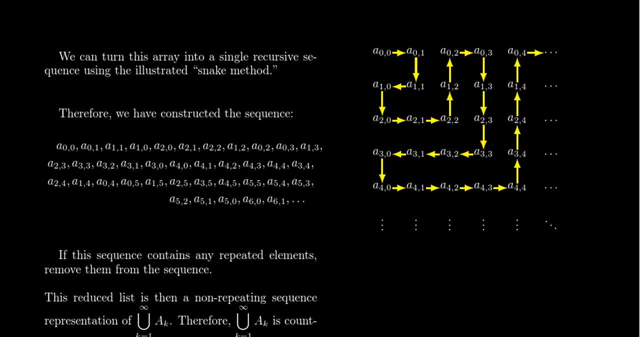 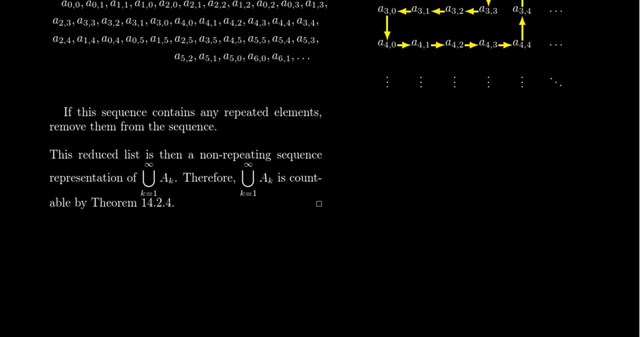 find the next number. Okay, This strategy will construct a non-repeating sequence, infinite sequence here. I guess with repetitions it might be finite. but whatever, Um, you are going to get a non-repeating list of numbers, finite or infinite. 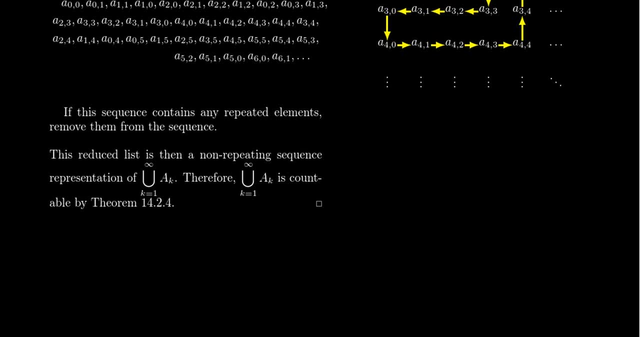 That'll then every element inside the union falls inside of that list somewhere And therefore by the theorem, we've proven this is a countable set, because we can list it all And again by similar reasoning. if you take an infinite- uh, an infinite intersection, this of course is a. 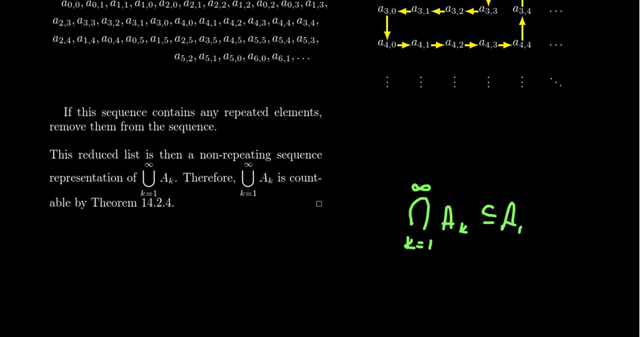 subset of a one, So it'll be countable. Um with intersections, you can take any intersection you want If you take a. if you take an uncountable intersection of countable sets, this will still be countable because they all sit inside of a one and subsets of subsets of countable sets are. 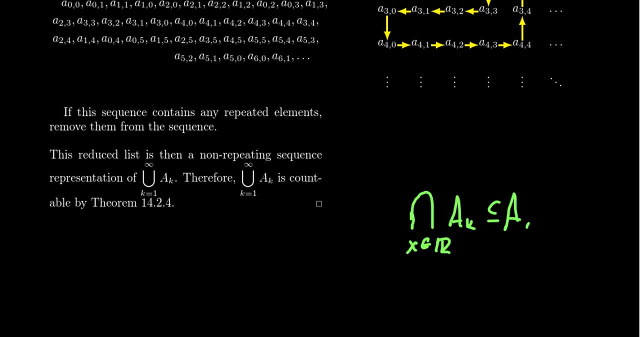 countable. So intersections are no problems whatsoever. If you take finite or countably infinite union sets, you're going to get a non-repeating sequence. If you take a non-repeating of countable sets, that does give you a countable set. If you take an uncountable union of countable, 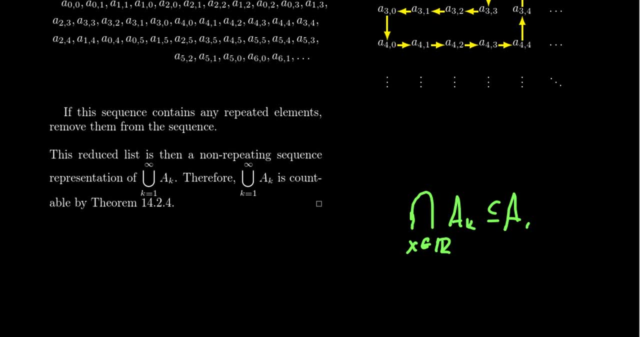 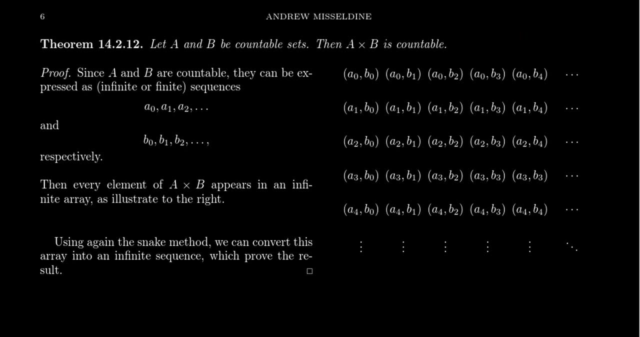 sets, then all bets are off. I mean, anything could happen in that situation. It could be countable, maybe, but most likely it would be uncountable. Another operation that we want to talk about here is Cartesian products. This gets a little bit more difficult, but sure enough. 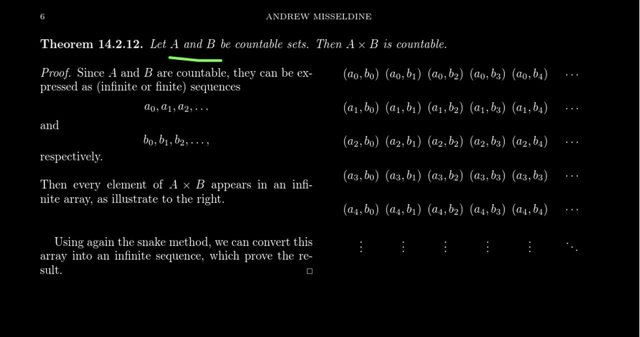 if you have two. if you have two countable sets, the Cartesian product of those two countable sets is likewise countable. The argument is actually very similar to the snake method We used on the previous theorem. So suppose we have two countable sets. They could be infinite. They. 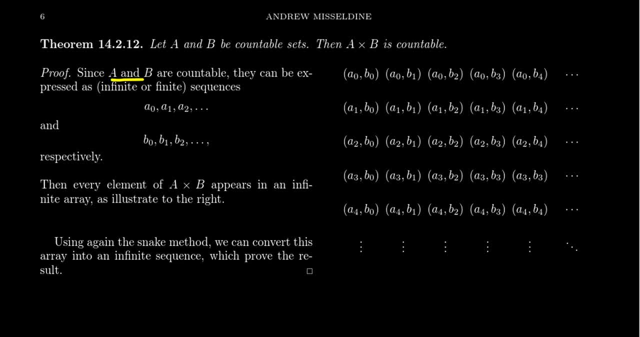 could be finite, Doesn't matter, Um, since they're countable. the elements of a can be listed: a zero, a one, a two. the elements of B can be listed as well: B, zero, B, one, B, two, et cetera. Then with: 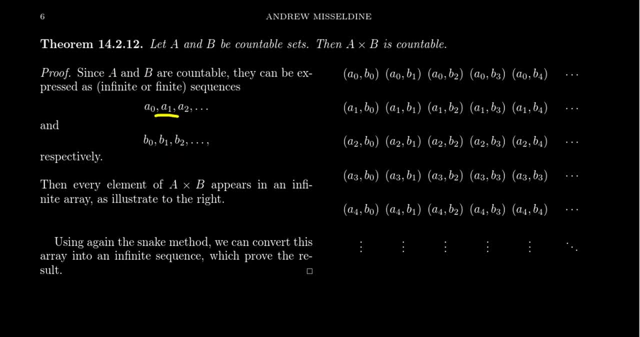 these two lists in mind, we can construct a two dimensional array that contains every element of a cross B, because a cross B is ordered pairs of elements. So you take an element from a and you pair it with an element Speaker 1 of B. you're going to use the elements of a to give you your first coordinate. You're going to 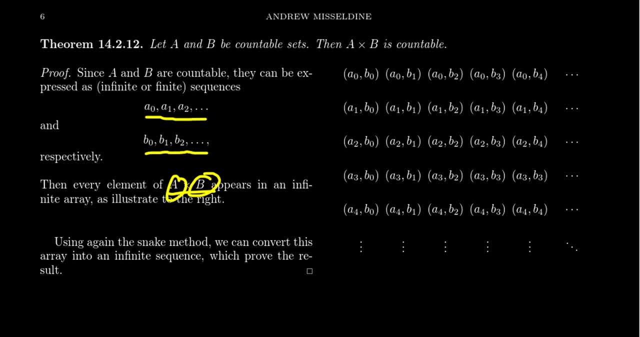 take the elements of B to be your second coordinate, And so, likewise, you construct this very large, most likely infinite, uh matrix again, for which you have the: a zero B zero a zero B one. a zero B two. a zero B three. a zero B four. a one B zero. a one B one. a one B two. 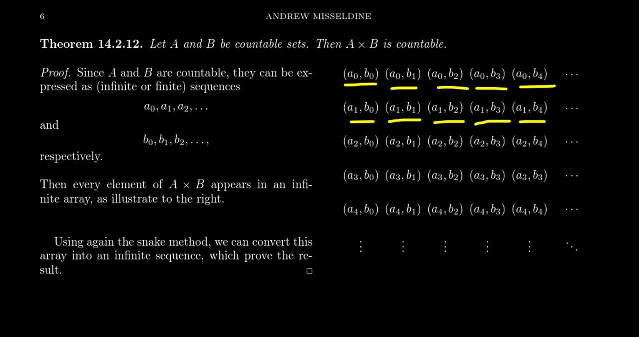 a one B three a one B four a two B zero a two B one a two B zero B two. You get the idea right, Um, using using the element elements, the index of elements from a as your first coordinate and index of elements for B, for. 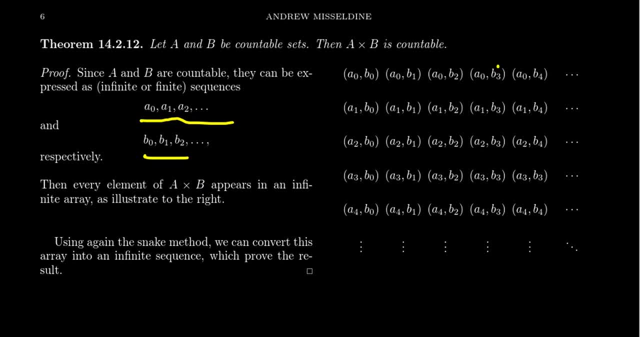 your second coordinate, we can then come up with another two dimensional infinite matrix that keeps track of all of the elements here. Every element inside of this, this set, shows up in this matrix somewhere, And so, using the snake method again, you can slither your way through this entire. 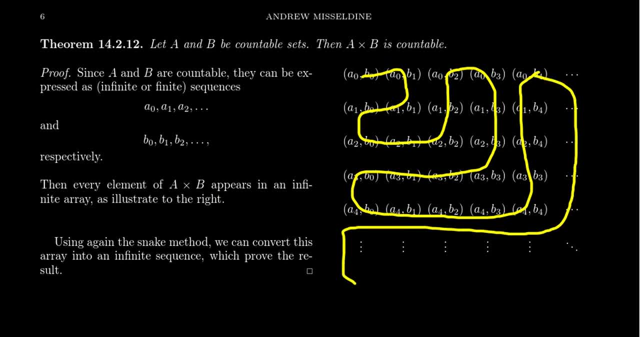 process and everyone's going to get hit If there ever is a repeat. um, that actually isn't going to happen here. uh, because, because this list is non-repeating, we can assume that this list is non-repeating, So none of the older pairs are ever going to repeat itself Now. 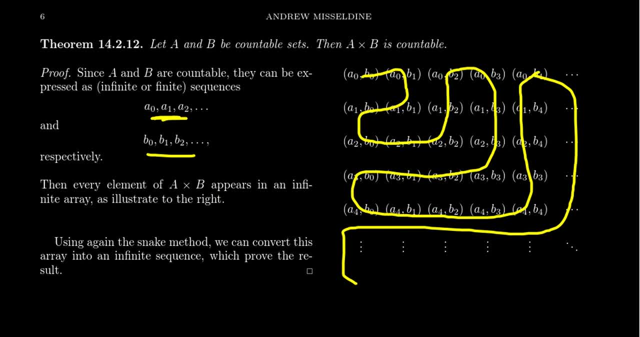 if this is a finite list, there might be a point where it stops this, because if there's any gaps, the snake will just jump over it. And if you, there might be a point where there's nothing left because maybe both sets are finite, That's fine. If it terminates, that's perfectly fine too. This. 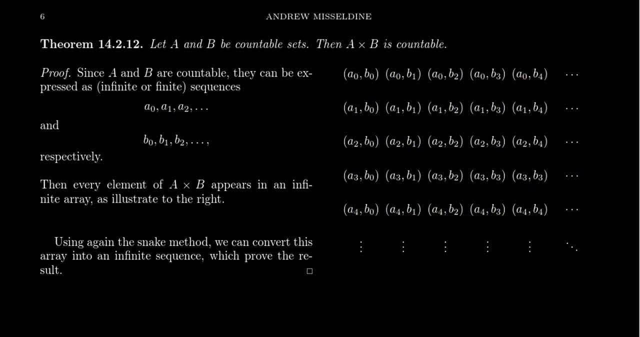 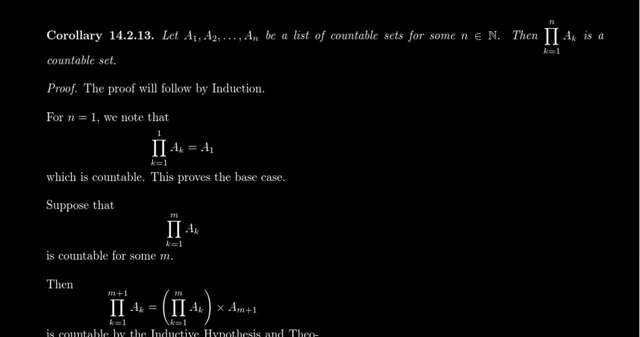 Using induction we can show that the finite product of countable sets is likewise countable. So if you have countable sets a1, a2 up to a, n and n is a positive integer right here- Then the product k1 up to n of the a ks is likewise countable. This is: 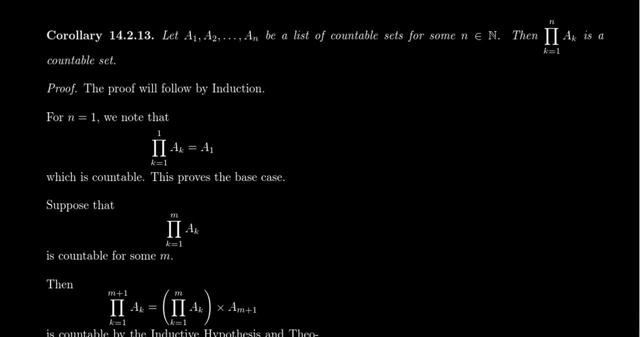 the exact same induction argument we did before The base case. When n equals one, you're taking a Cartesian product of just one set. That'll just give you back a1 itself, um, for which that was countable. Now I'm going to mess this up a little bit. I'm going to do a little bit more. 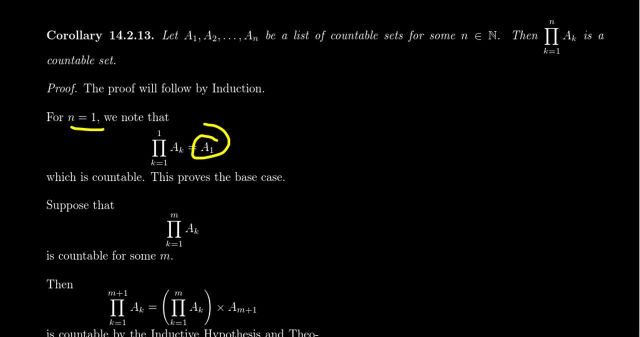 countable by assumption. so that gives us the base case again. your base case is really zero, in which case if you take the product of nothing, you go back to the empty set. uh, that of course, is also a countable set. so whichever base case you decide to use, it's going to be just fine, no big deal. 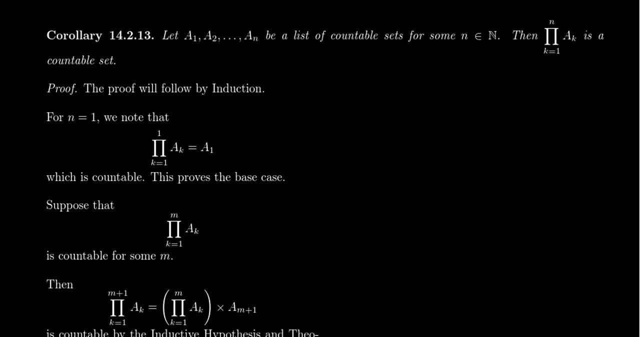 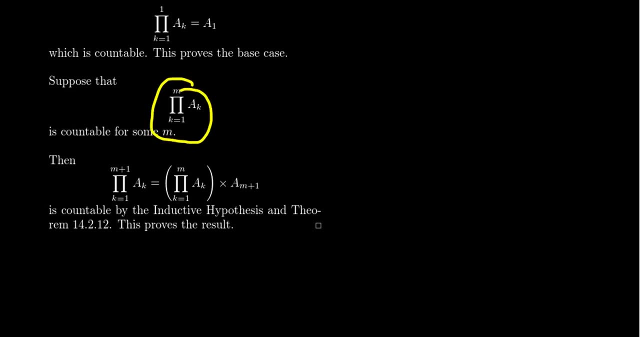 uh, people don't typically talk about empty products, but it's, it's relevant to mention there. so then your inductive hypothesis: assume you take the m-fold product, cartesian product of countable sets, assume that's countable. then look at the m plus one fold cartesian product. 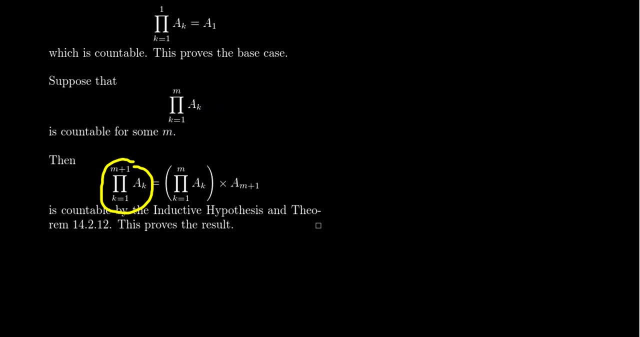 well, the m plus one fold cartesian product is the m-fold cartesian product times the next, the next function there or the next set, excuse me, m sub m plus one. by assumption, a m plus one is countable by our inductive hypothesis. the m-fold cartesian product is countable there and 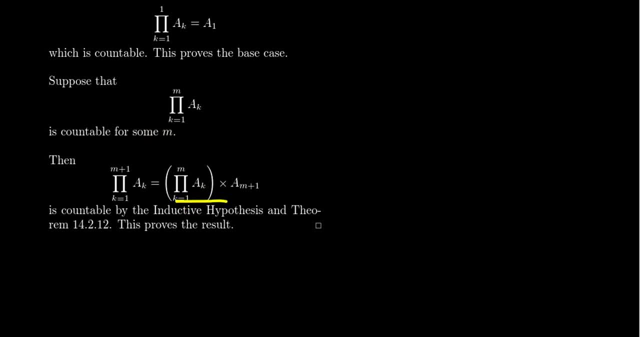 then we just previously shown that the, the cartesian product of two countable sets, is itself countable, and therefore this gives us that the m plus one fold cartesian product is countable. so any finite cartesian product of countable sets is countable. so if i took for 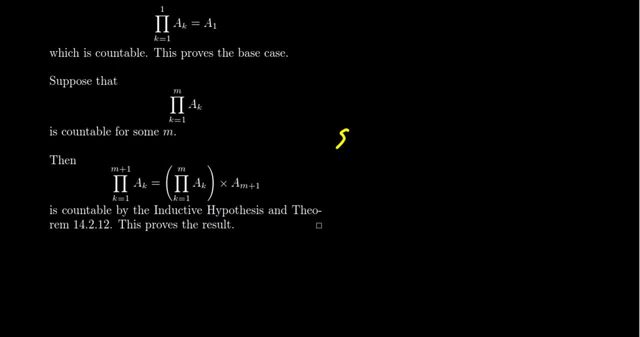 example, um, the set zero, one cross the natural numbers. this is a countable set. it's countable, uh, because you took a countable set cross a countable set um. you could even take, for example, n cross n, then this would likewise be a countable set. 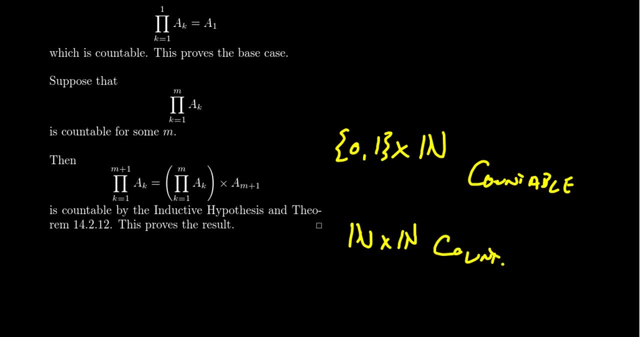 And you can come up with more exotic ones as well. On the other hand, though, you have to be very cautious. This is about as far as we can go here, because, unlike the theorem we saw above about countable unions, the corresponding theorem for Cartesian products is false. 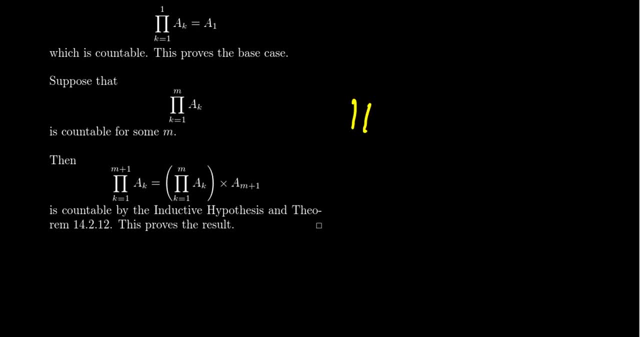 That is to say that if you take the Cartesian product where k ranges from 1 to infinity of a sub k, this set is uncountable. Now with the unions, if you take a countable union of countable sets, that is countable. 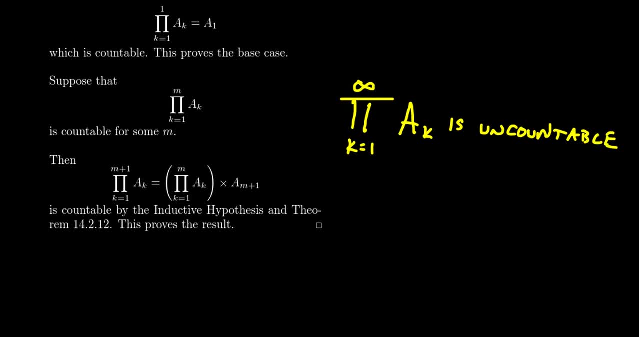 But the countable product of countable set is actually guaranteed to be uncountable, And this is an example we're going to explore more in the next lecture. here We're actually going to look at the set. take the set of binary sequences. 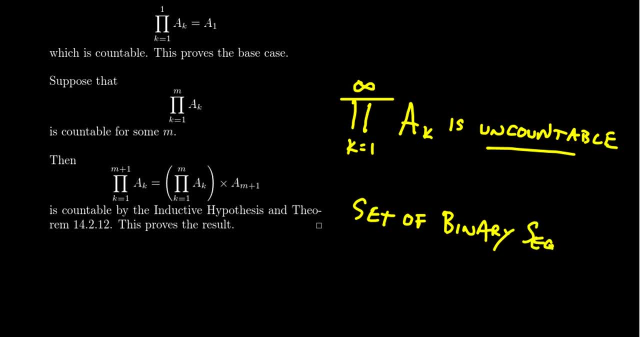 That is to say, if you have a binary sequence, this would be something like 0, 1, 1, 1, 1, 0, 0, 1, 0, 1, 1, 0,, etc. 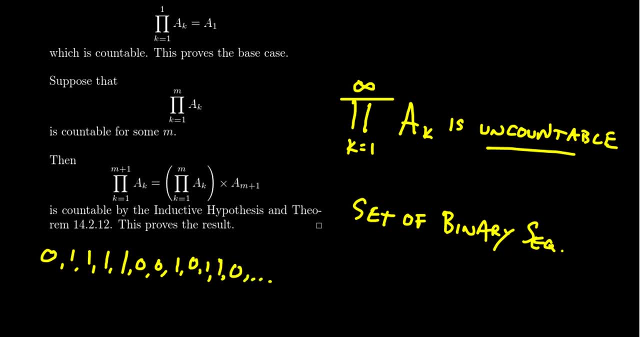 So this is an infinite list of numbers that consist of only 0 and 1s. If you take the set that contains all of these things, this set we are going to see is actually uncountable. It's an uncountable set. 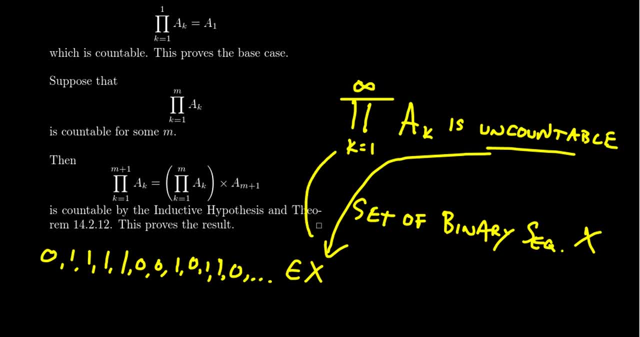 And this set, of course, is actually an example of such a thing. This set X is actually equal to the infinite Cartesian product, where K goes from 1 to infinity. here of the set 0, 1.. So you can identify a sequence as an infinite Cartesian product. 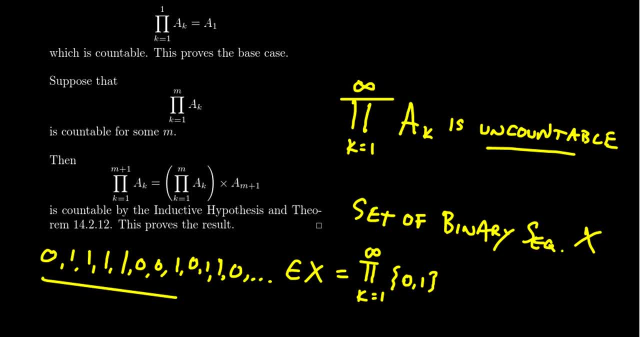 Because, after all, what is a sequence? It's an infinite list. Order does matter. So if a Cartesian product gives you ordered pairs, a threefold Cartesian product gives you ordered triples. a fourfold Cartesian product gives you ordered triples. a fourfold Cartesian product gives you ordered quadruples. 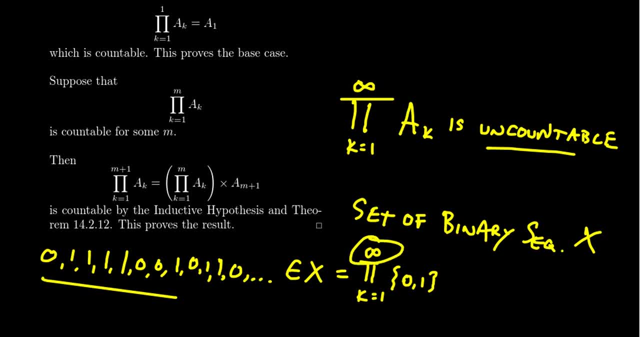 And so an infinite, accountably infinite Cartesian product is actually going to give you sequences. And so if you take the infinite product of the set 0,, 1, and you do this over and over and over again, right? So in some respect this is the set 0, 1 to the infinite power. 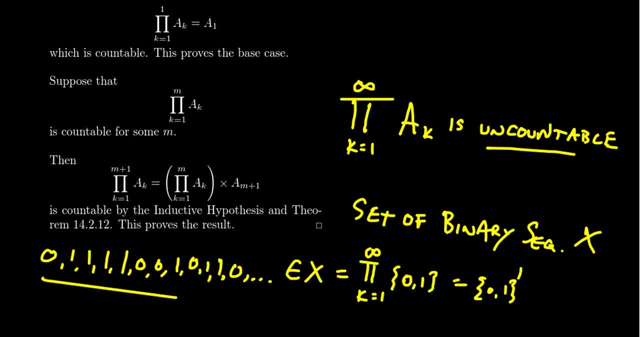 More precisely, this is the Alof, not power. there. This actually gives you an uncountable set. We're actually going to show that this set has the same cardinality as the power set of the natural numbers, But again, we'll talk about that more next time. 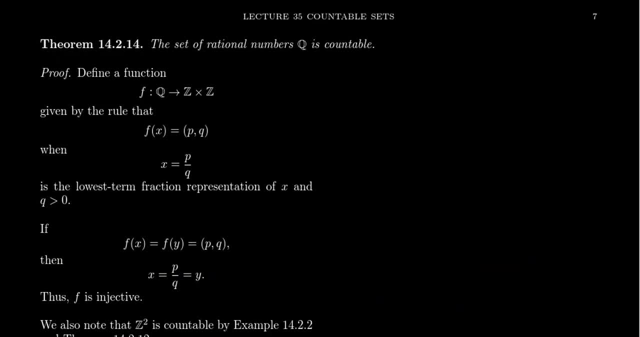 Before we end this video, there is one other important example. I want to mention the rational numbers. We've talked about the integers. The integers are countable. The natural numbers are, of course, are countable by definition, But the rational numbers are likewise a countable set. 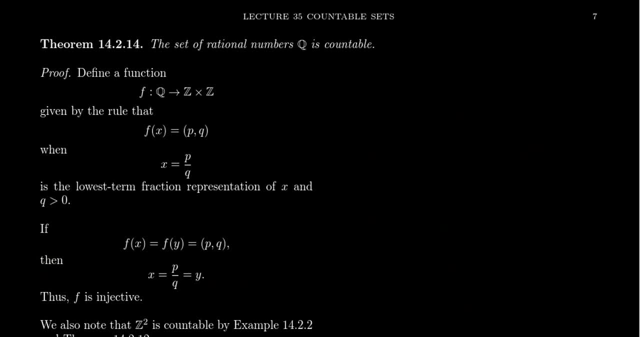 That one's a little bit hard to believe Because if you look at it in terms of the geometry of the real line, right, Okay, we got the integers. I can see that. So you have like 0,, 1, but between any two integers there's a gap. 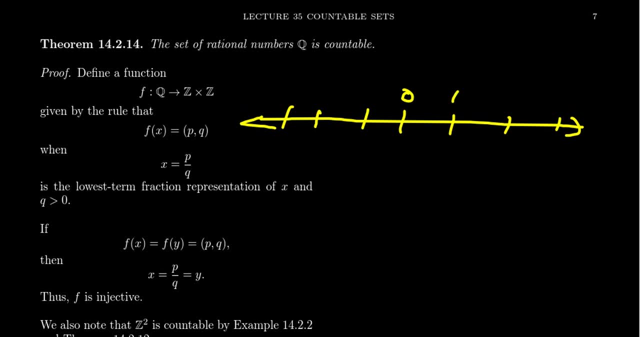 There's not any integers between 0 and 1.. That's what makes these things discrete. On the other hand, with the rational numbers, between any two rational numbers there's another rational number and another one, and another one. So, honestly, between any two integers there's infinitely many rational numbers, right. 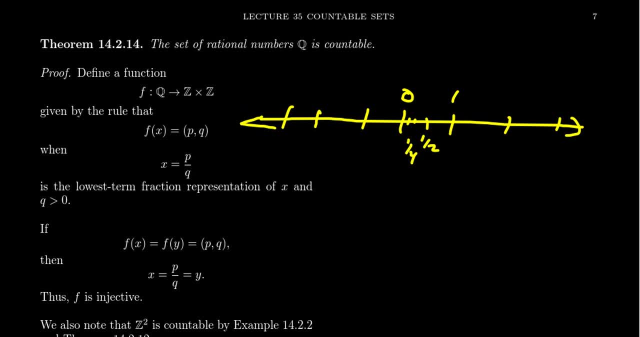 So the terminology we use here is that the rational numbers are dense, that between any two there's always another one. So given any like any interval of rational numbers, there's infinitely many rational numbers inside of that set. You can't do that with integers. 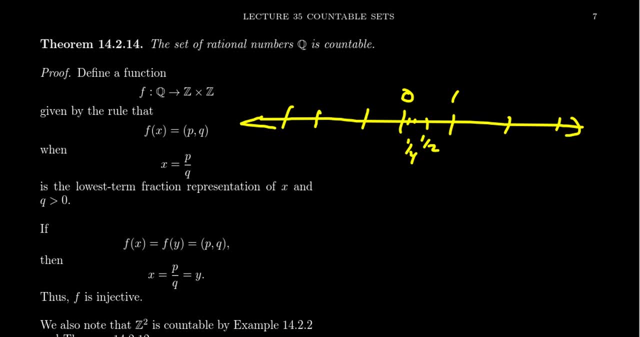 Integers have gaps, They are discrete, But the rational numbers, on the other hand, are dense. So in some regard one can make the argument that there are more rational numbers than integers. But that's actually a falsehood, At least when we're talking about cardinality. 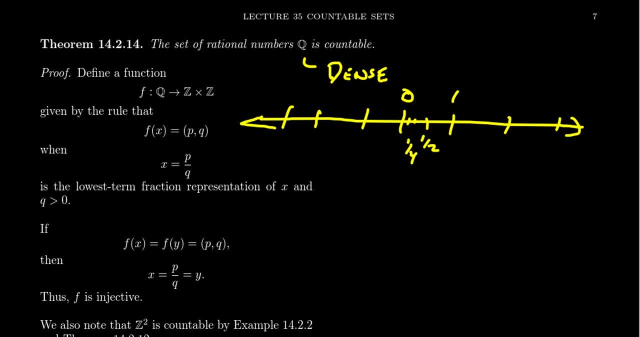 Like we had mentioned before, if you're talking about like measure or geometry, maybe there's a geometric notion, an analytic notion or a topological notion of size, But if we're only talking about set theory, we're talking about cardinality. 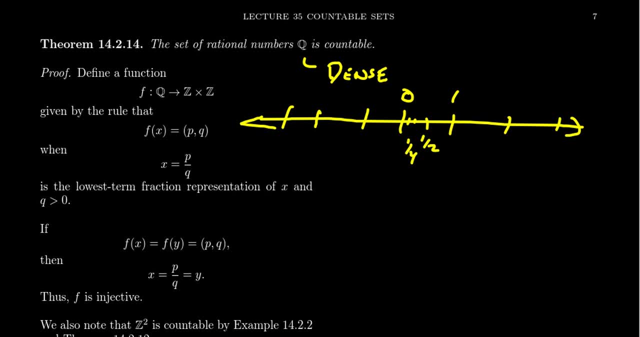 And the cardinality of the rational numbers is the exact same as the natural numbers. This is a countable set, And the way we're going to do this is the following: We're going to construct a function, f, where f is a function from the rational numbers to z cross z. 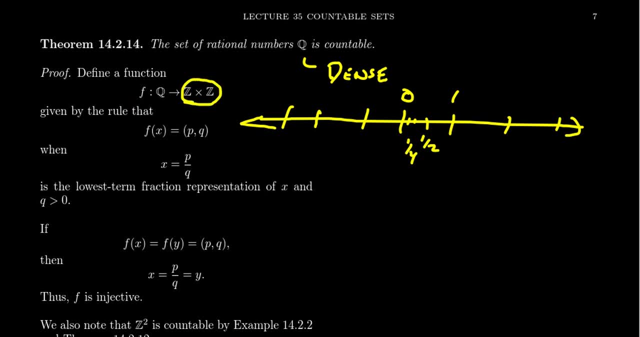 I want you to be aware that z, cross, z is a countable set. How do I know that? Well, z is a countable set. We came up with a specific bijection between the natural numbers and the integers. And as we go along, 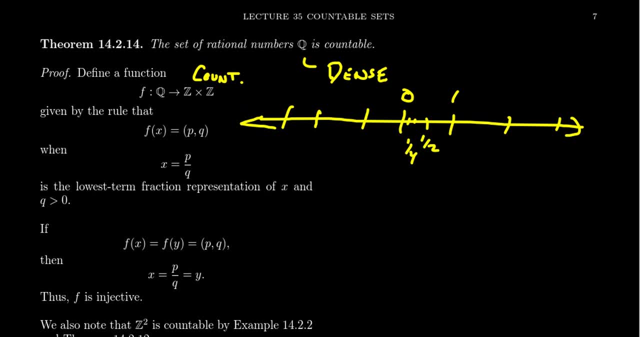 as we just have seen, the Cartesian product of two countable sets is countable. So this is a countable set. Now we have a function between a set, the rational numbers, with a countable set. Well, what's the formula here? 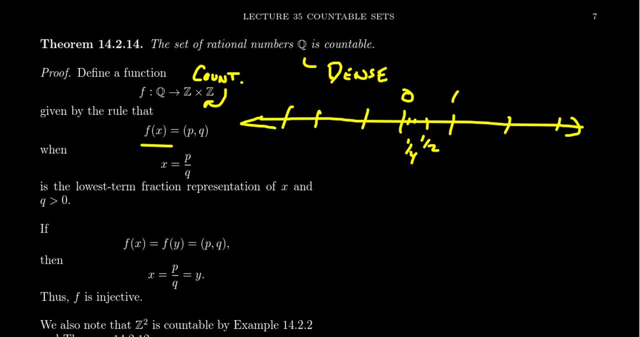 Where, if you take any rational number x, I want you to take f of x to be the ordered pair p comma q, where x is equal to p comma q And p comma q is the lowest terms. So, for example, if x equals one half, 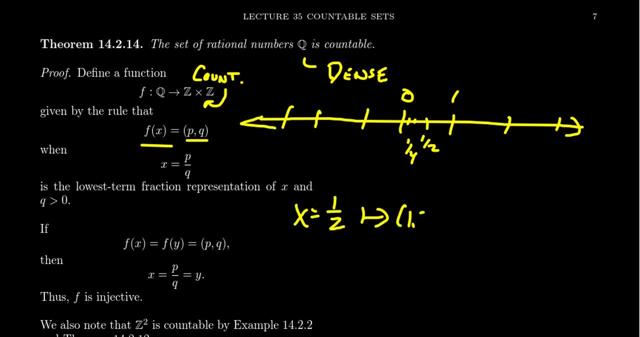 you're going to map this over to one comma two. If x equals three, you're going to map this over to three comma one. If x equals zero, you're going to map this over to zero comma one. If x equals negative three halves. 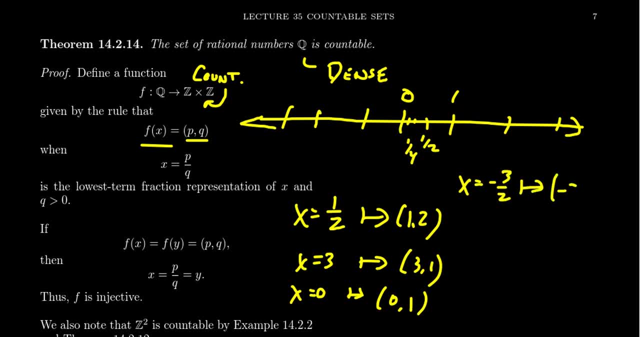 you map this over to negative. three comma two: You always assume the denominator is going to be positive. You can always make that assumption. This is in lowest terms. There's no common divisors between the two terms there. That is, the numerator and denominator have a gcd of one. 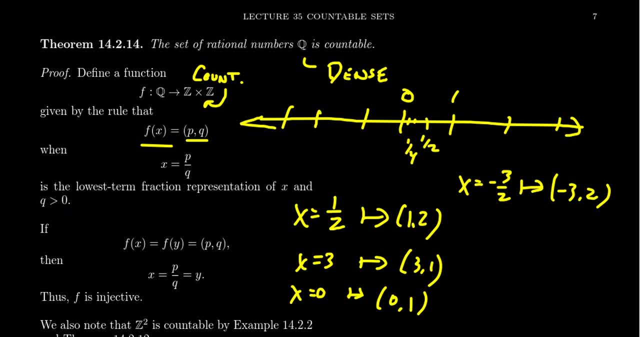 Such a number always exists and this is unique for every rational number. So if you use the lowest terms representation, this is well defined as a function. So this is a function. Is it one to one? Well, if f of x equals f of y, 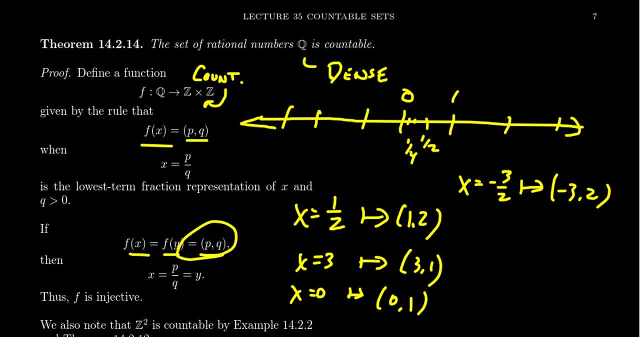 that means their image is the same. So there's some p and q. Well, if f of x is p comma q, that means x as a rational number is equal to the fraction p over q. But likewise if f of y has the same image, 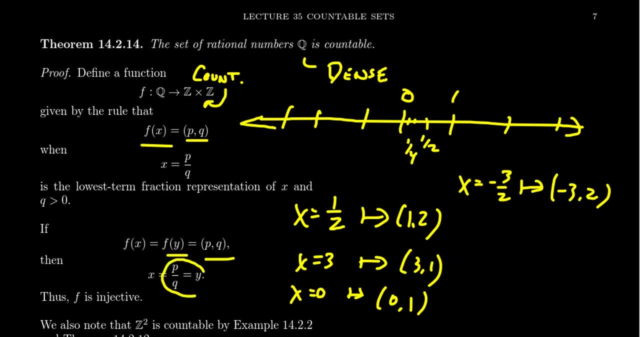 that means y as a fraction, as a rational number, is equal to the fraction p over q, Since they're the same fraction, they're the same rational number. So that's injective, And I should mention that one of the corollaries we mentioned earlier in this lesson. 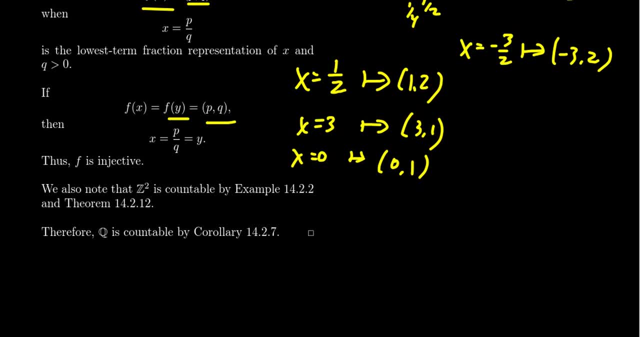 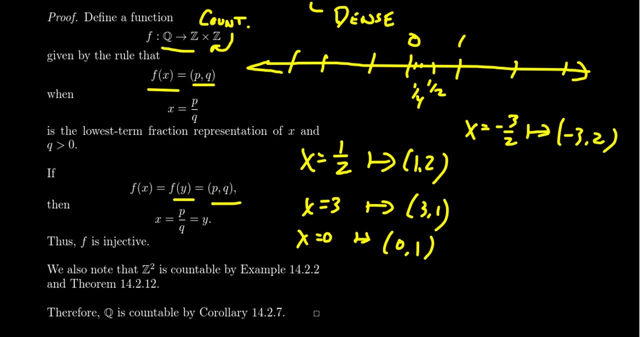 said that if you have a map, let's look at this again. If you have a map from a function to a countable set, that is injective, that corollary guarantees that this thing is the domain- is countable as well. 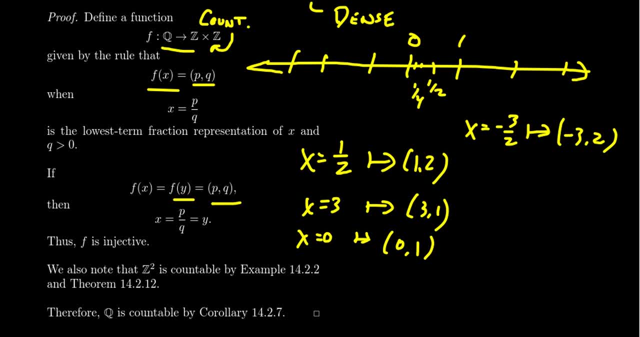 So because we can inject, we can embed the rational numbers inside of a countable set that makes themselves countable. Now you could also prove the rational numbers is countable directly using a snake argument that we did before, And if you want to, 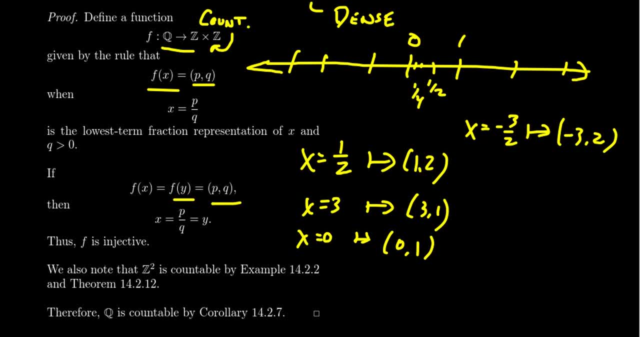 I'll leave that up to the viewer to do that, But this gives us some examples of some very important countable sets and operations that you can do with countable sets to retain the countability of the set In our next lesson, which will actually be the final lesson for this lecture series, number 36,. 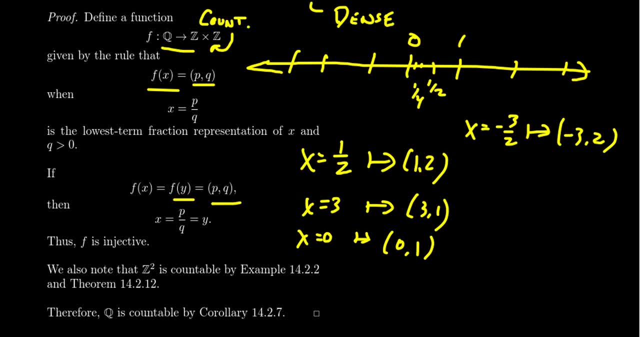 we'll talk about uncountable sets and some of the consequences to set theory and advanced mathematics. But that brings us to the end of lecture 35.. Thanks for watching. If you learned anything about countable sets in this lecture, please like the video. 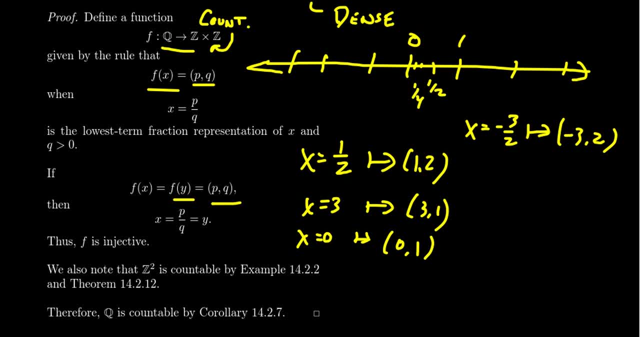 Subscribe to the channel to see more videos like this in the future. Refer this video to friends or, you know, colleagues who might be interested in this as well And, as always, if you have any questions, feel free to post them in the comments below. and I'll be glad to answer them as soon as I can. 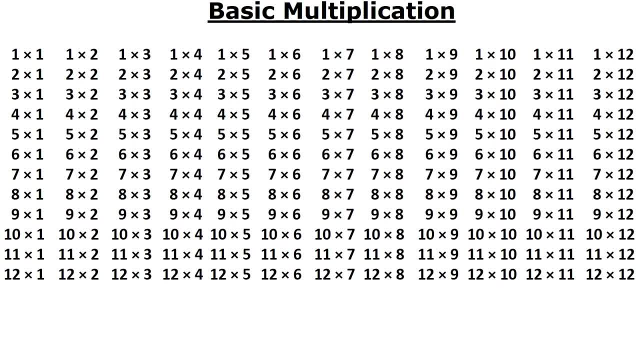 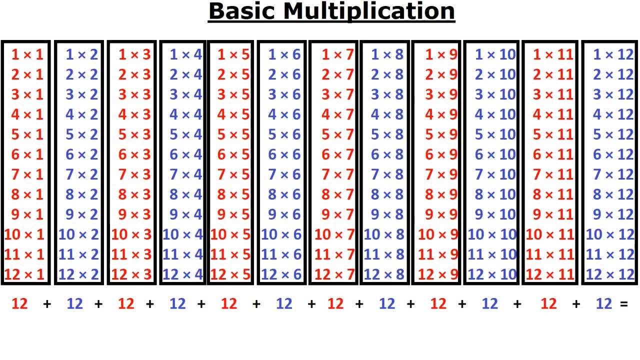 In this video, we're going to take a look at how, at Math TA, we've created the fastest, easiest and most efficient way for students to learn their multiplication tables. So, right off the bat, from 1 x 1 to 12 x 12, that's a total of 144 multiplication tables. That's 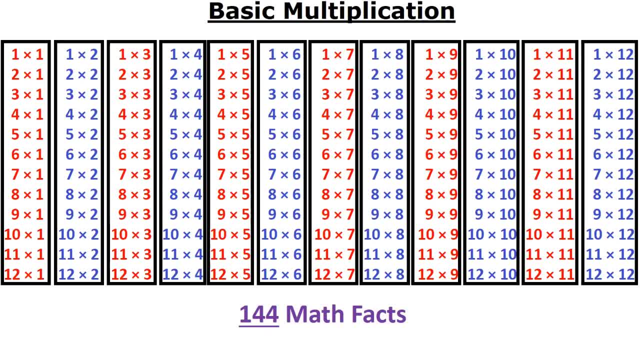 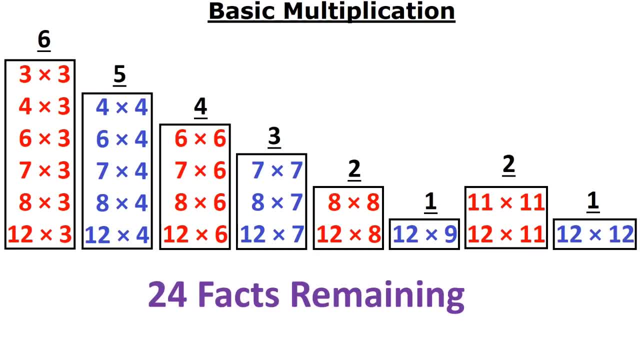 a whole lot of things to remember. However, we've created a method where, if you just know 6 rules, just 6 rules, you can go from 144 down to only 24 remaining. That's right, from just 6 rules, we go from 144 Math Facts down to 24.. How is that possible? Well, let's take 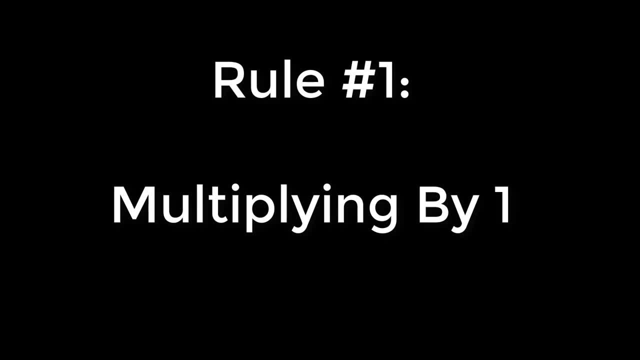 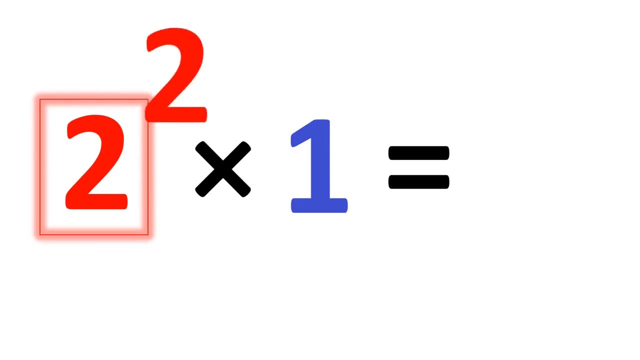 a look. So we begin with the easiest multiplication rule to remember, which is multiplying anything times the number 1.. Anything times the number 1 is that number 1 x 1 is 1.. 2 x 1 is 2.. 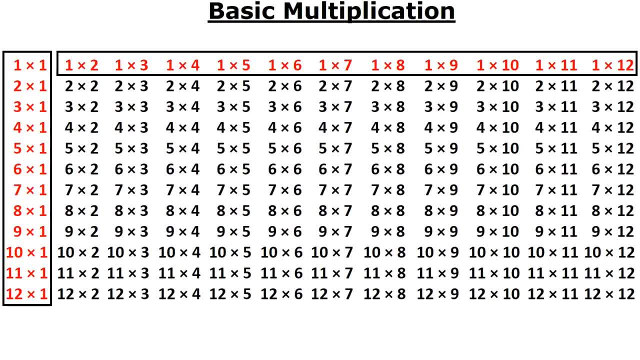 3 x 1 is 3, etc. Well, you also know the reverse. You also know 1 x 2,, 1 x 3,, 1 x 4.. So from that one simple rule, you actually know 23 Math Facts. The next rule is multiplying.